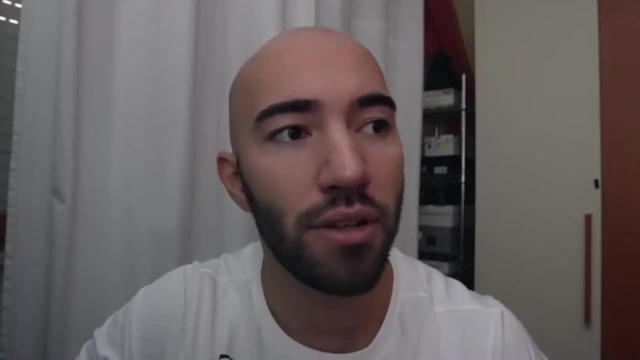 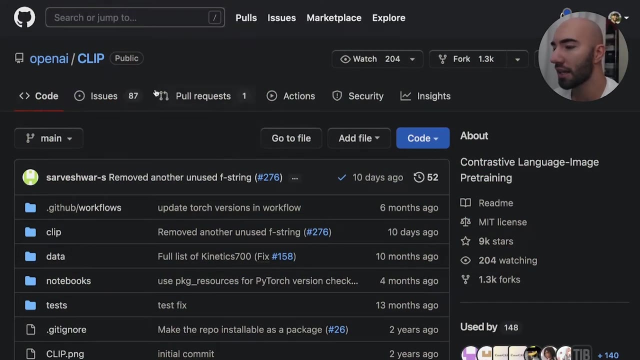 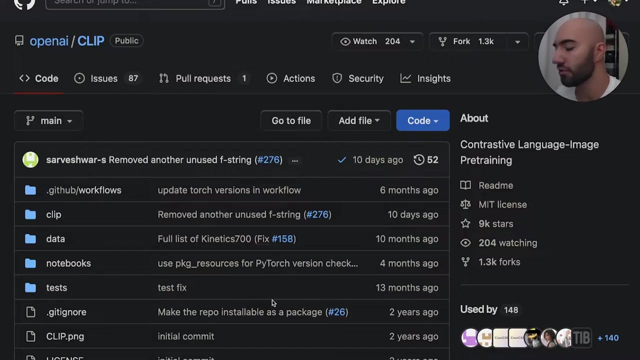 There's a good chance. We can do it with clip. So let's have a look at how we actually use to clip opening. I released a github repository Open. I clip here. this contains Clip, but we're not going to use this implementation. We're actually going to use this implementation of clip. 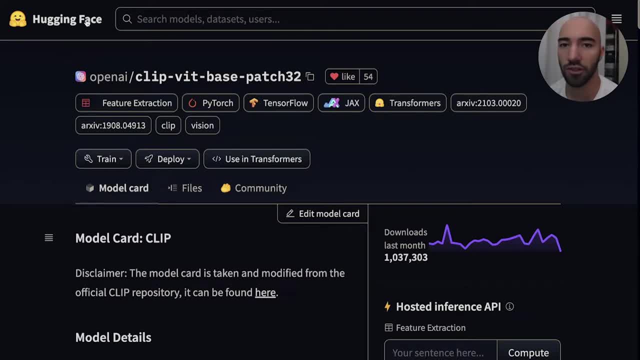 So this is on hooking face, So we're gonna be using hooking face transformers And this is still from open AI, It's so clip, It's just an easy to use implementation of it through the hooking face transformers library, Which is a more standard library for actually doing anything with with NLP and also now so computer vision. 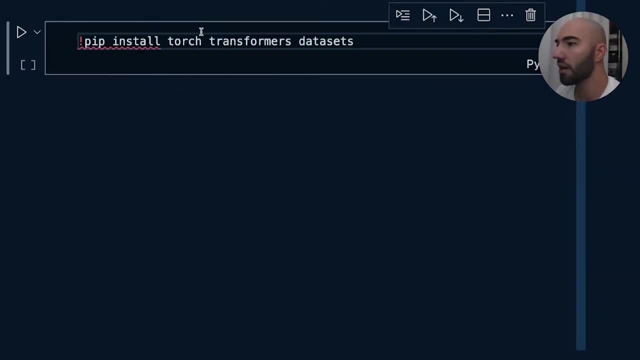 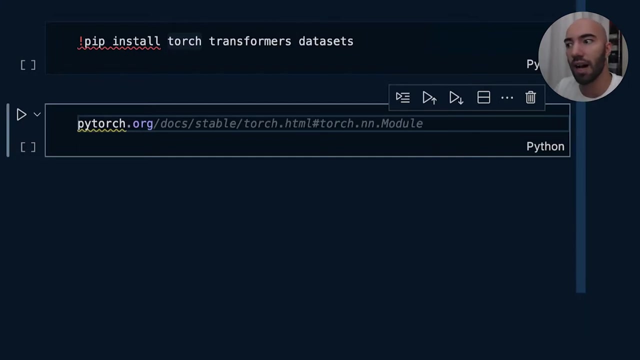 And some other things as well. So to get started, I'd recommend you install these libraries: pip: install torch. you should probably go through the PyTorchorg instructions rather than following this here. so go to PyTorchorg and just install PyTorch using the. 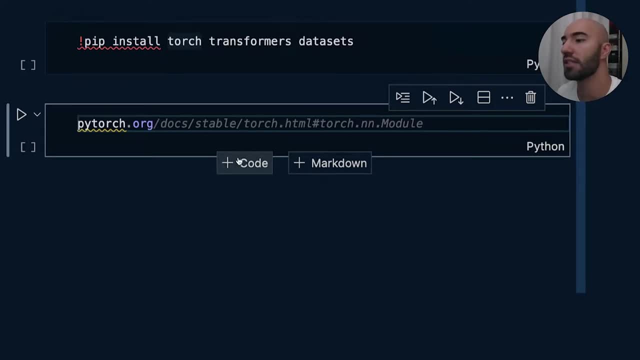 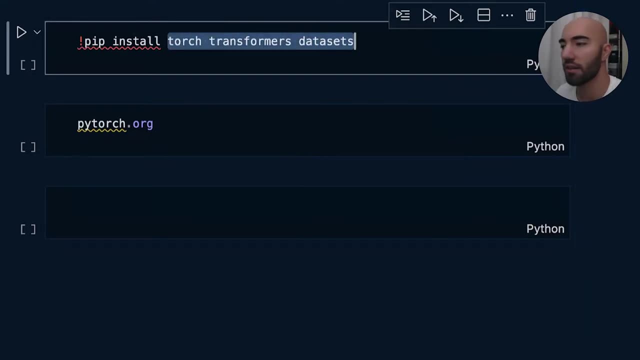 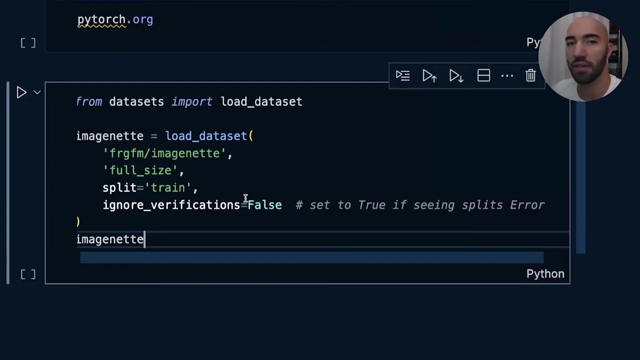 Specific install command they use for your platform or your iOS From here, and then they've installed transformers and datasets. you can, you can, so just use this command. So I'd recommend installing PyTorch from here instead now. after that We're gonna need our, our dataset. 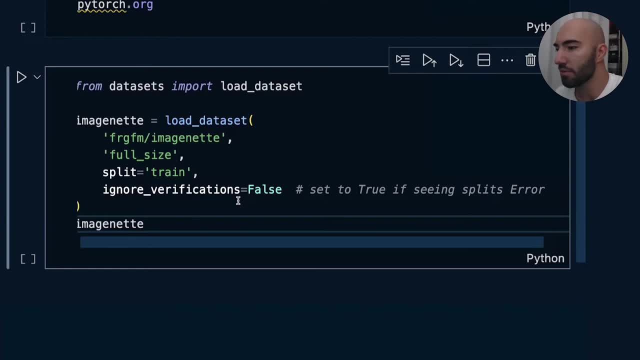 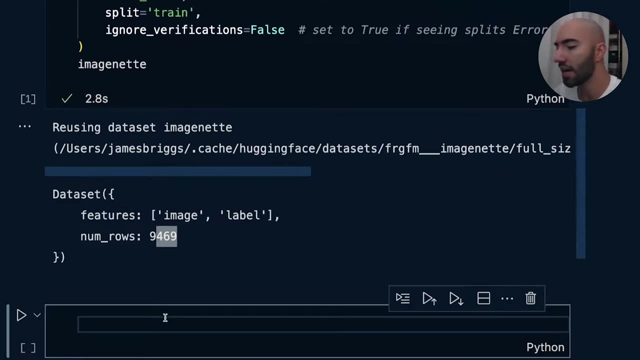 Okay, so this is just a very simple dataset. it Contains, I think, 10, just under 10,000 Images and we only care about the images here. So if we have a look, we have image, net Will go the first item. we'll just have a look at image. 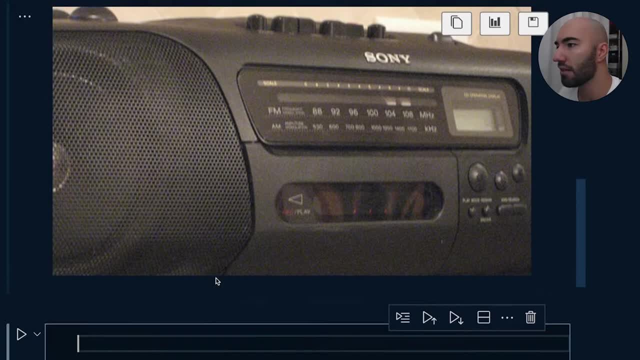 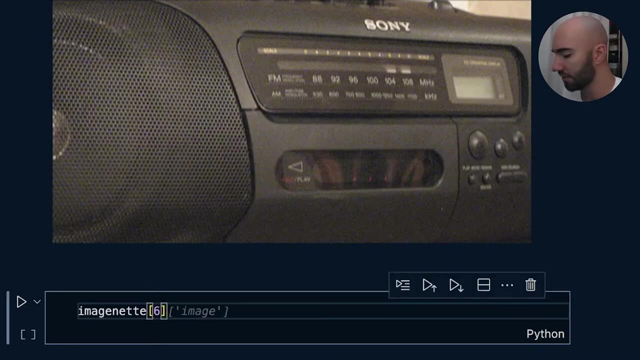 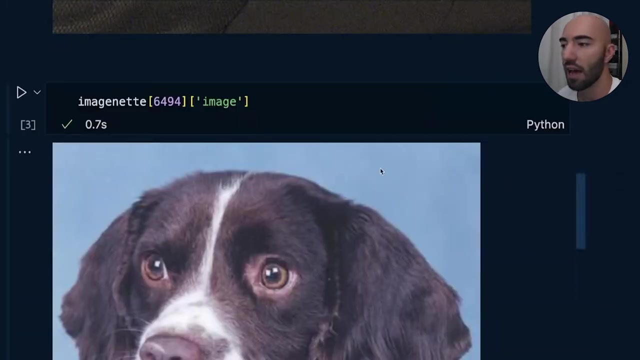 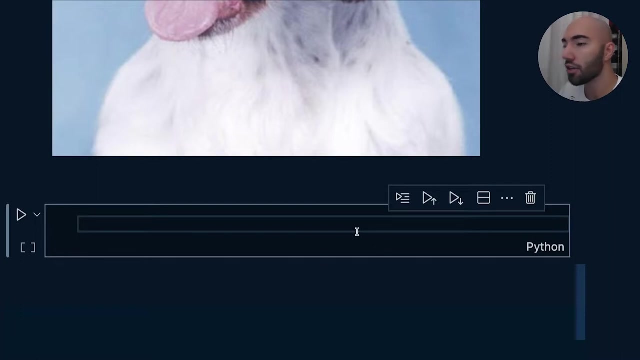 Okay, and we have this like Sony radio, And we have other things as well. So, if we go image net, Kate's six, six, four, nine, four. there's another image here of a dog. okay, just to point out that we have a lot of images in here in this data set that cover a range of things. um, there are, there's not a. 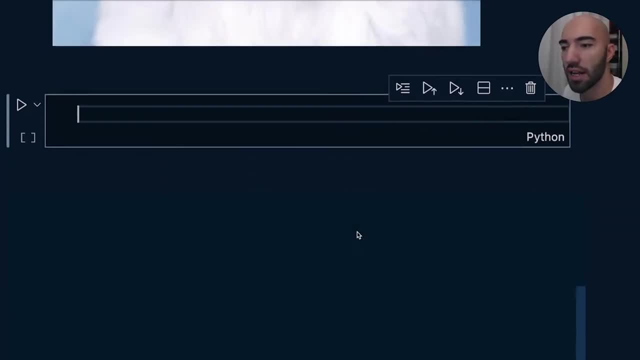 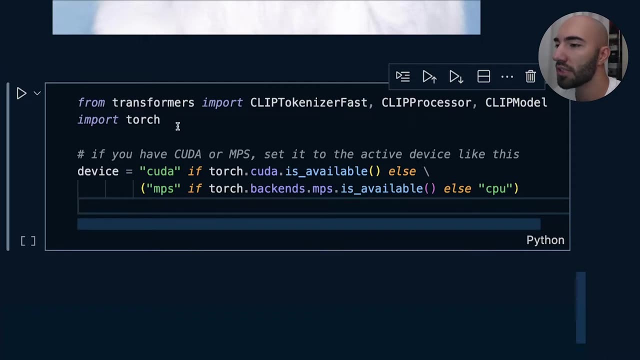 huge number of different categories here, but they have dogs, they have radios and a few other things. now i'm just going to go ahead and initialize everything. so there's a few things here. from transformers, we're importing the clip tokenizer, so the tokenizer is what's going to handle the 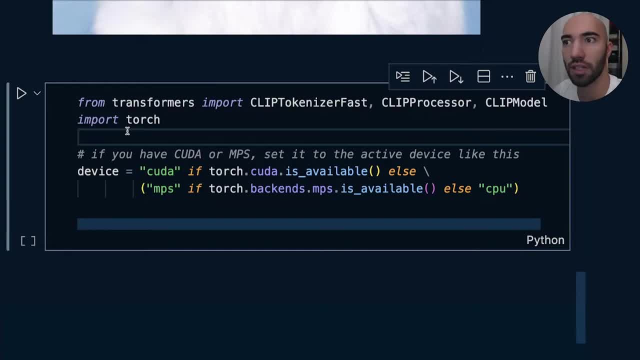 pre-processing of our text into token id tensors and other sensors. we have the clip processor. that's like the, the tokenizer, but for images. so this is actually just going to resize our images into the size that clip expects and also modify the picture or values as well. and then we have clip model. clip model is is clip itself, okay. so, uh, if you. 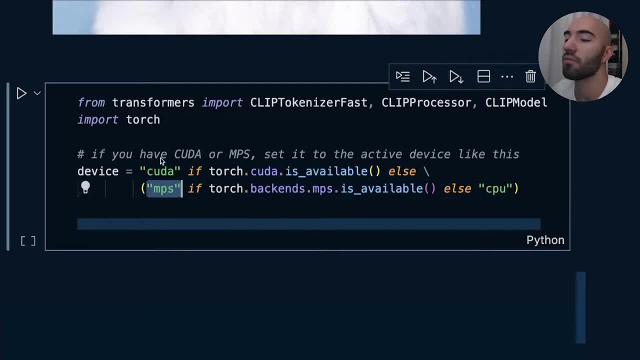 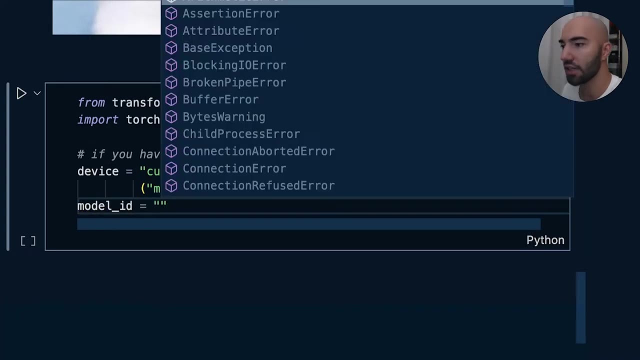 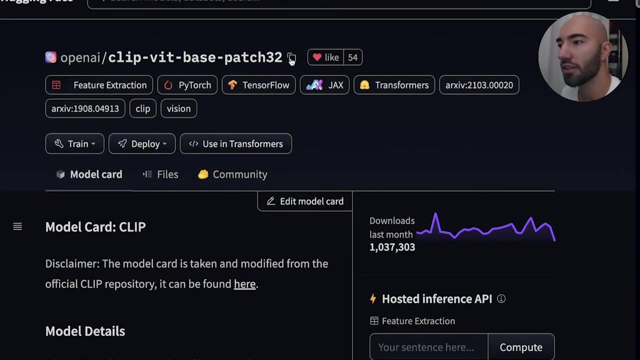 have cuda or mps. if you're on m1 mac, you just set that with with this, okay, um, and then we're ready to actually initialize all of this. so, uh, the model id is going to be what we saw before. so you come over over here. we have this open eye clip vit base patch 32 copy. that. 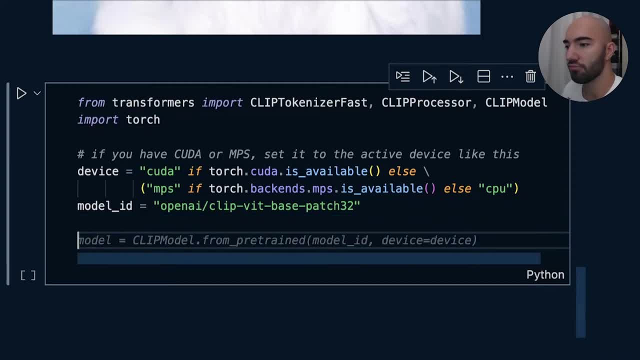 and here we go, okay, and now we just need to look. i'm being told what to do already, okay, so model clip, model from pre-trained uh, model id i'm going to. i don't normally set device like that. i don't know if you can, i am going to do it like this, okay, and tokenizer: okay, good job. 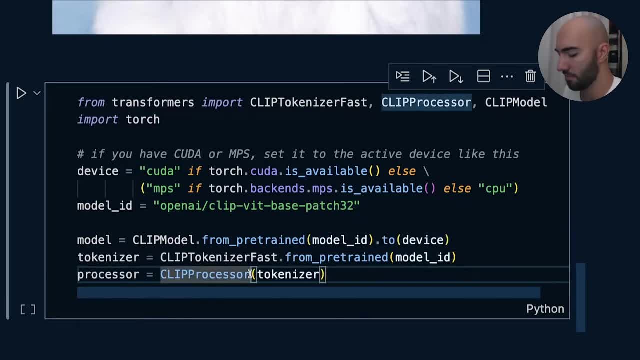 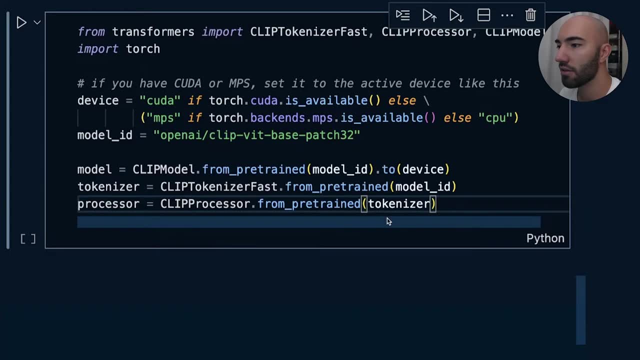 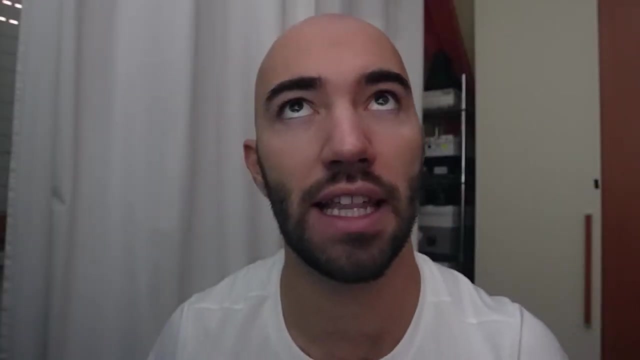 and processor: cool, almost there it's before. i'm pre-trained. okay, um and oh, you got a little bit confused, so model id: okay, that looks good, let's run that. okay, cool. so now what we're going to do is take a look at how we actually create the, the text embeddings through clip. so we start with prompt. 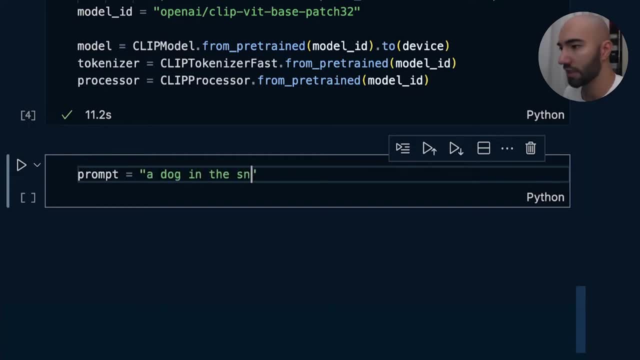 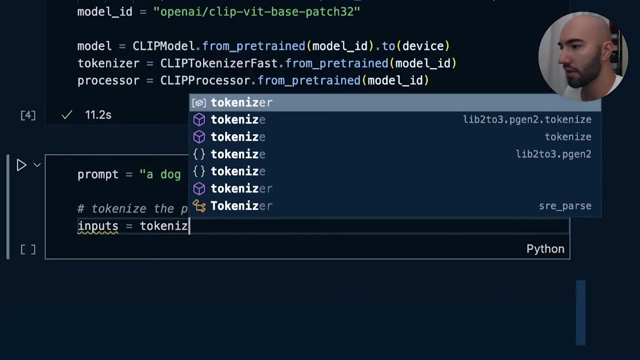 i'm going to go with a dog in the snow. there's not many pictures of dogs in the snow in the state set, but there are some- and what we need to do is is tokenize the prompt. yep, that's true. okay, and i'm not going to do it like that. we're going to go with tokenizer prompt and the we need to. 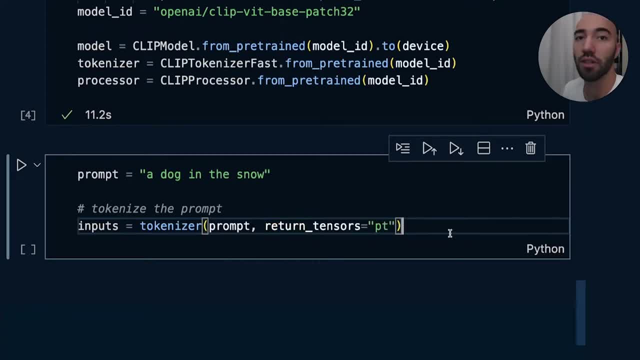 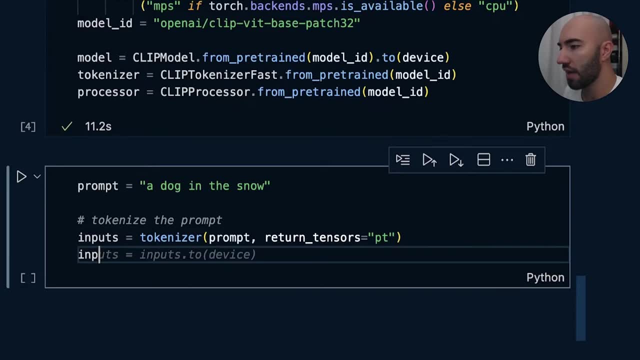 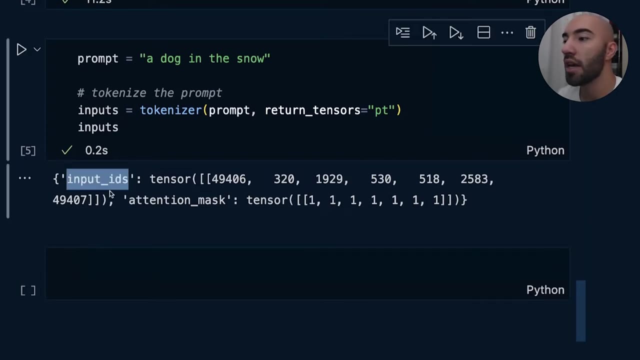 return tensors using pytorch. so we're using, we're going to be using pytorch behind the scenes here, um, so make sure we do that. and let's just have a look at what is actually in inputs. okay, so we get the. this input id is tensor, so you'll, you'll recognize this, uh, if you, if you use hugging face transformers before. 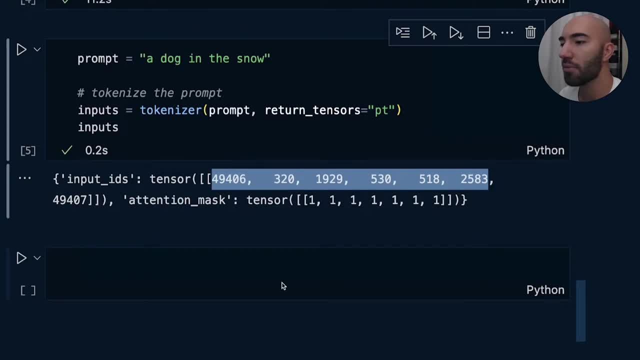 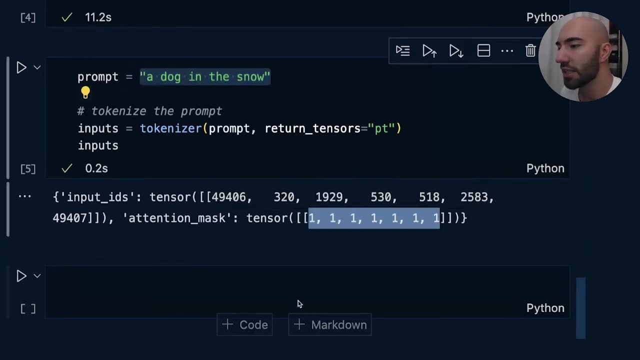 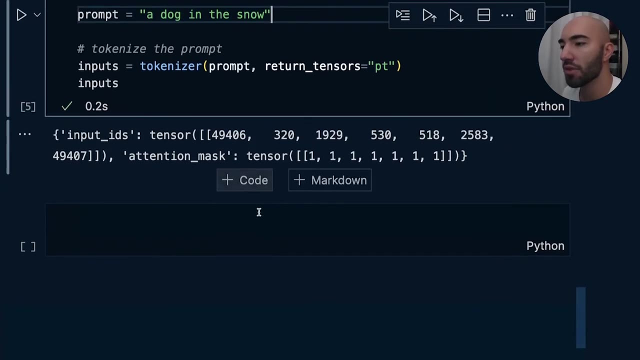 uh, these are just the id token ids that represent the words from this. okay and these. this is the attention mask now for us. it is going to all be ones, but if we had padding in here, the length of our prompt would become a zero, telling the model to not pay. 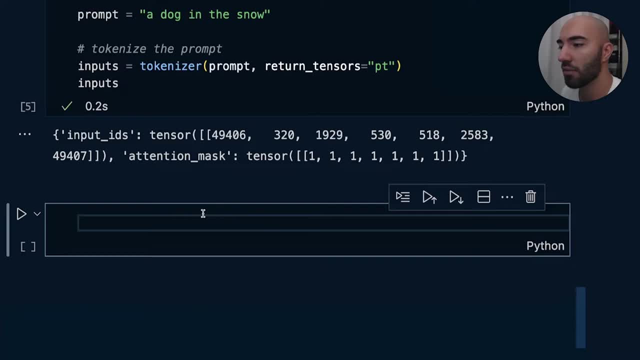 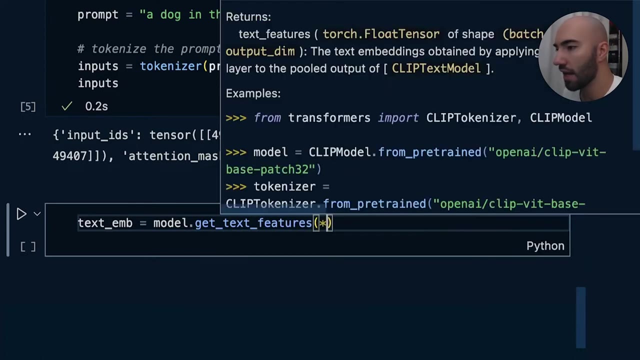 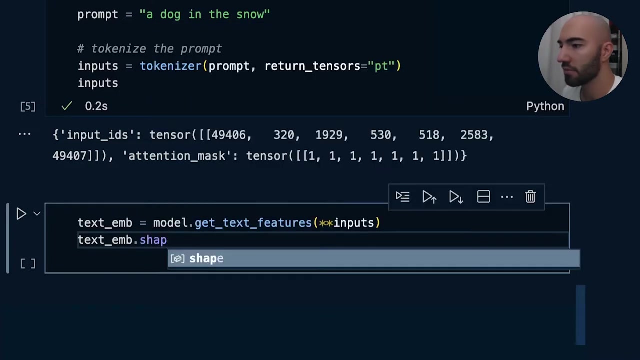 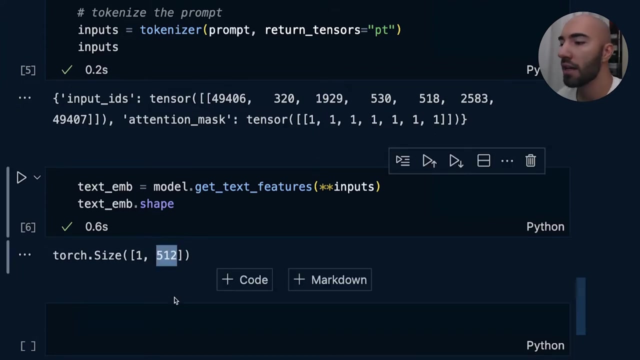 attention to to that part of the prompt and from there we can process this through clips. so we do model, get text features, I think, and we pass in those inputs. okay, and let's have a look at the shape of that. okay, so we have a 512 dimensional vector. okay, so that's the text embedding side of things. 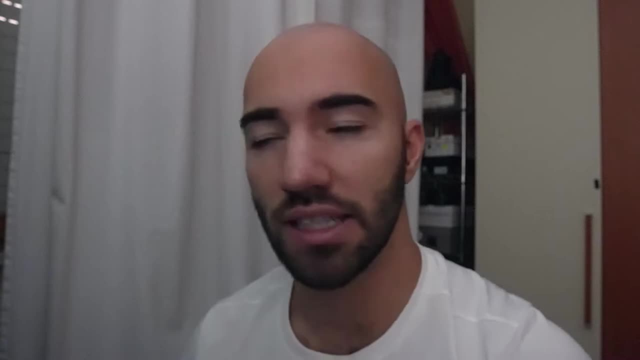 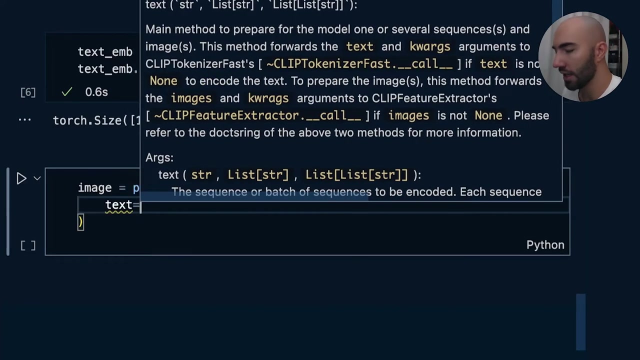 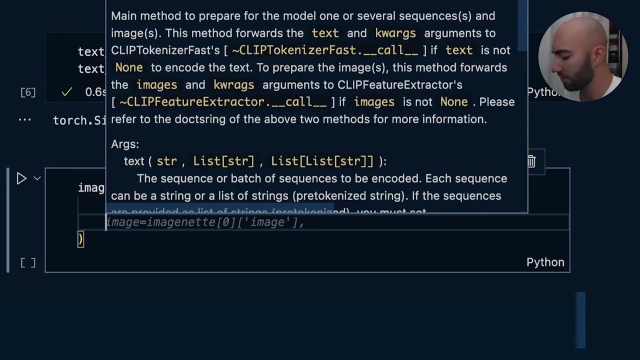 now we need to go ahead and do the image embedding side of things. okay, so we're gonna resize the image. first the processor. we're not adding any text in here, so you can also process text through this processor. I'm just keeping it separate because it makes more sense to me. the image should. 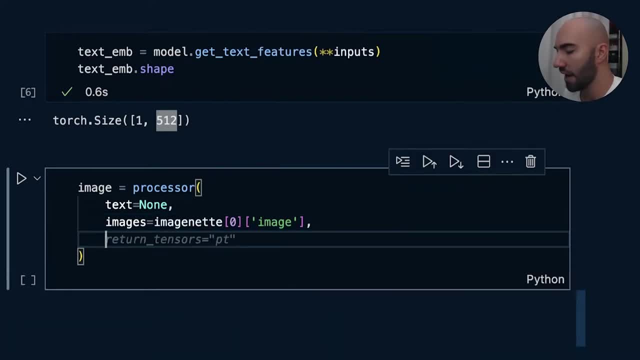 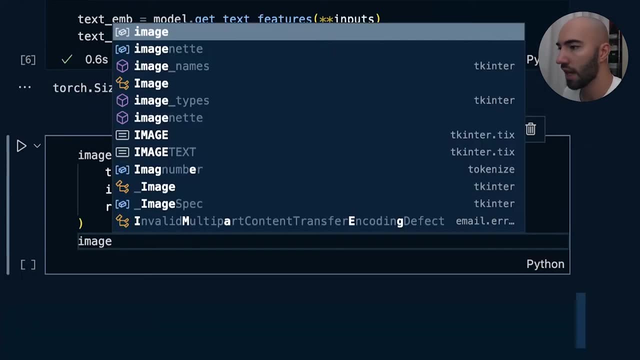 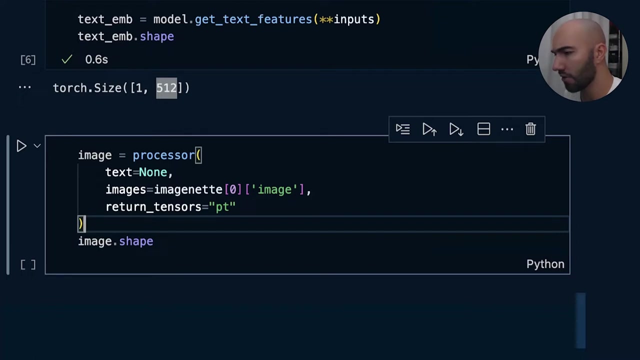 be images. actually, again, we want to return sensors using pie torch, okay, and then we can have a look at the. I'm gonna, I'm gonna show you the image. first, we just have a look at the shape and as well. one thing, so, okay, I can show you. 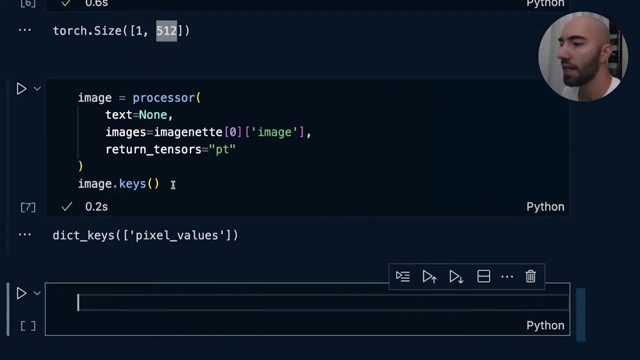 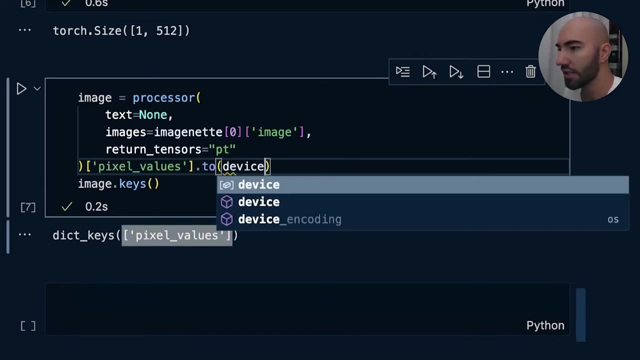 okay. okay, in here we actually have this pixel values, so we actually need to extract that. so we're gonna put it here. I'm gonna move those to the device as well. I think the device I have self right now is actually CPU, so it doesn't make a difference for me, but that's fine. so let's have a look at the shape, okay. 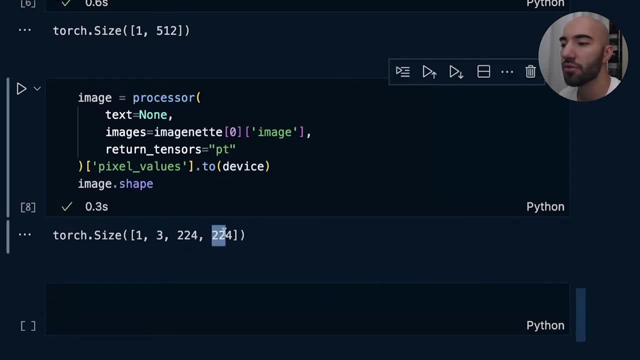 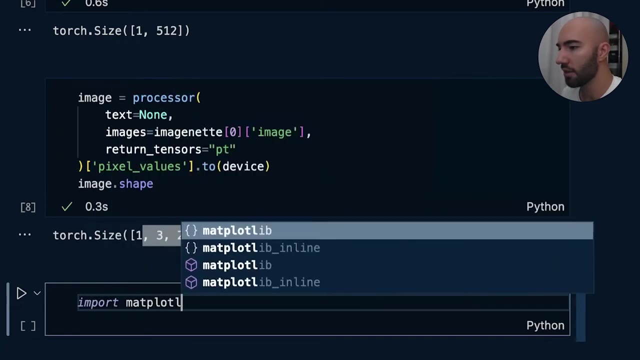 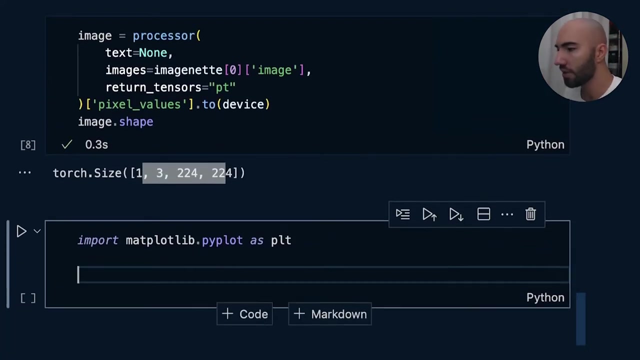 so you see that we have this 124 by 224 image with three color channels. so this is just the expected shape that will be consumed by the vision transformer of clip. okay, and to import matplotlib pie plot PLT, and I just want to show you this image. so this: 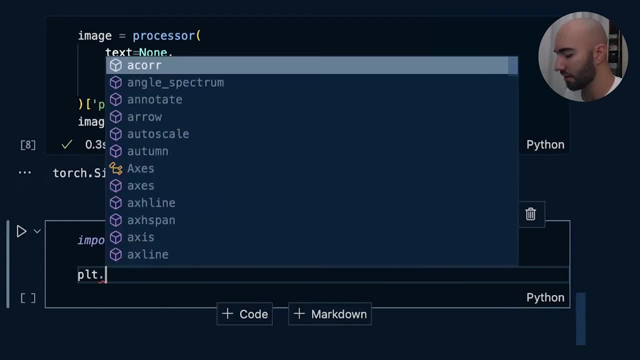 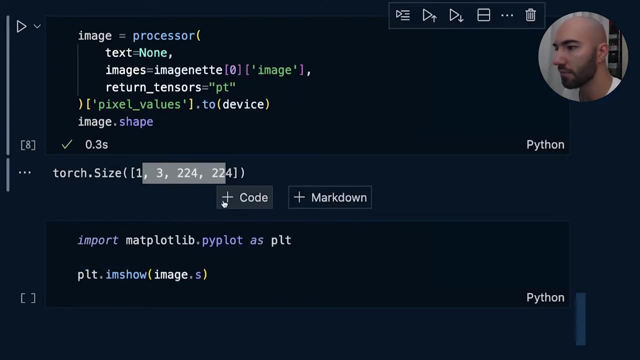 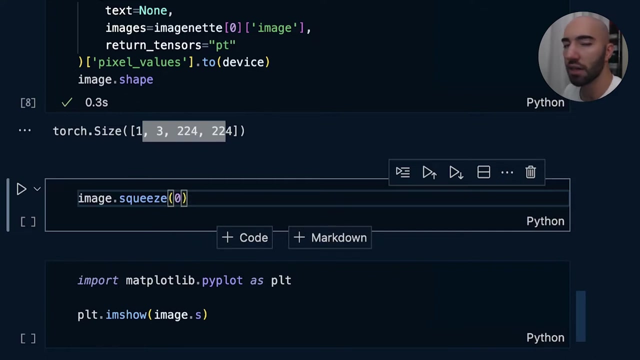 resize image. so yeah, see, I'm show and I need to, so I just need to resize it. let me show you what I'm actually doing here. so image dot squeeze zero. so I'm gonna remove that first dimension. now I'm going to transpose it. so we put the three color channels at the back and 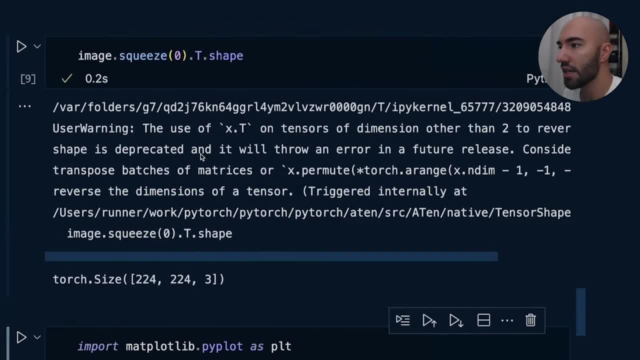 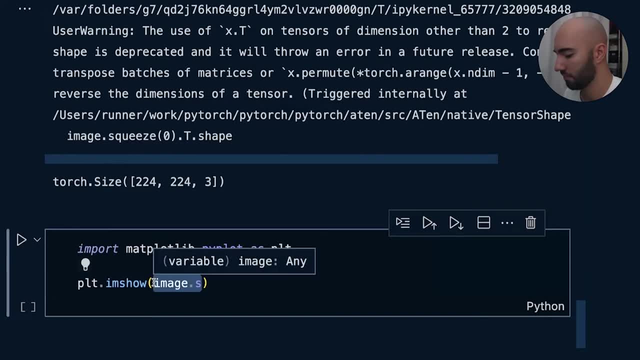 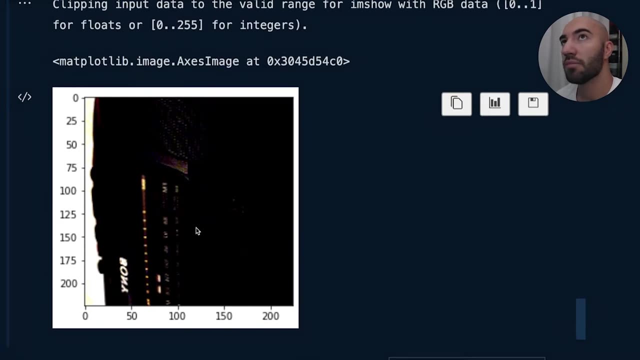 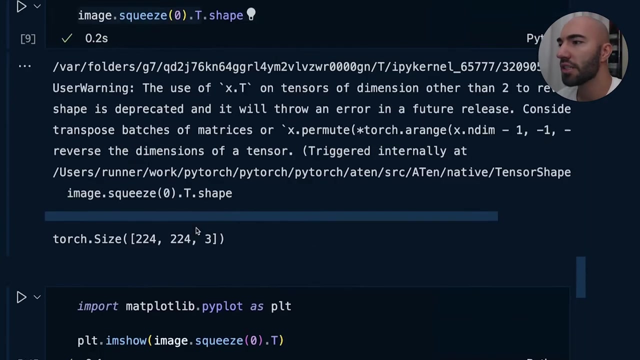 this is for. this is for matplotlib to be able to actually show us this. so I'm gonna take that, I'm gonna put it here, okay, and you can see. so the the minimum maximum color values are all of the color values. pixel values are modified when we do this, process it through the 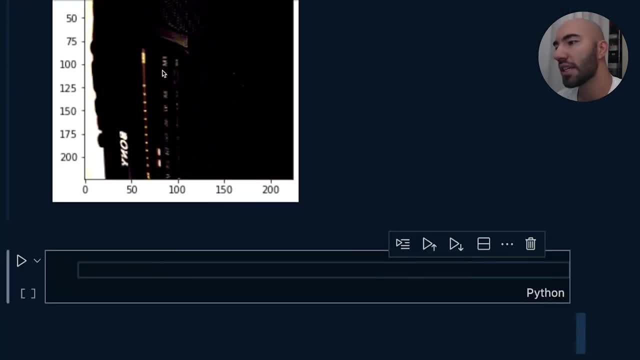 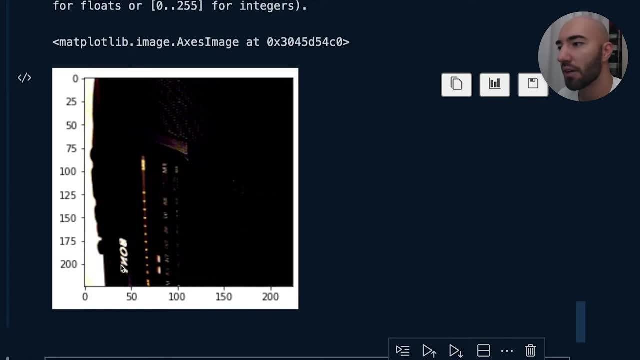 processor, so the colors are kind of messed up, but you can see that this is like a resize. you know what we saw before? okay, we can still see it's a Sony, just kind of backwards now and flipped. we can saw that. see, that is that Sony radio. 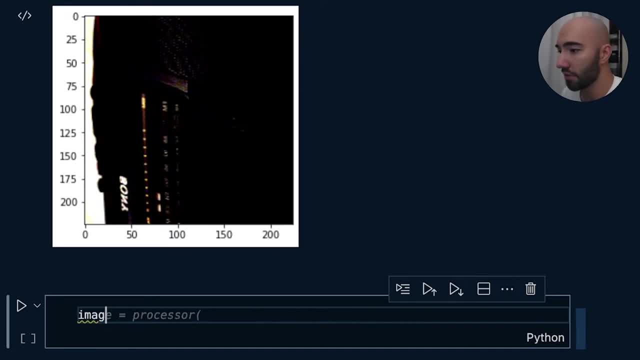 okay, and then we just need to go over to our softwares and see if we can actually see this image. so I'm gonna go over to image check and I'm gonna click the image and I'm gonna click the image check and select image and you can see. 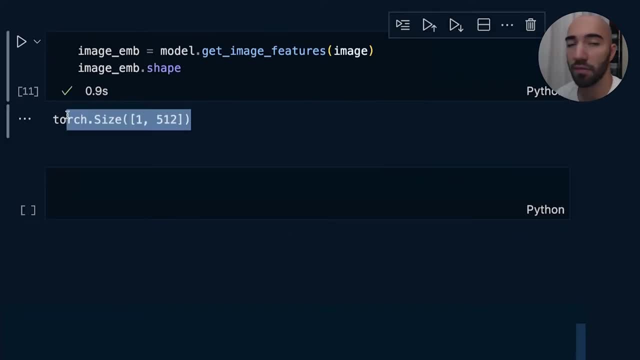 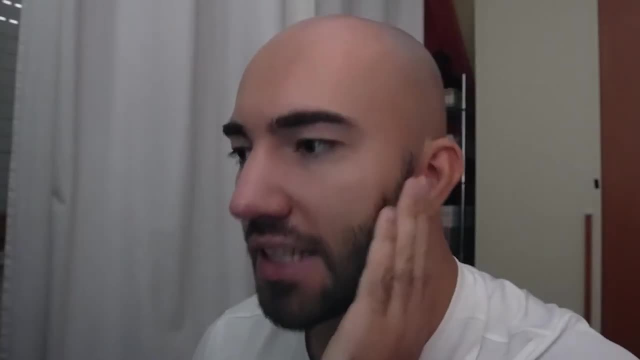 that it's showing the model and the image and um, you can see how I can change this image a little bit. you can see it's the same as the previous one, so you can actually see like I have an image here and you can see how I changed the. 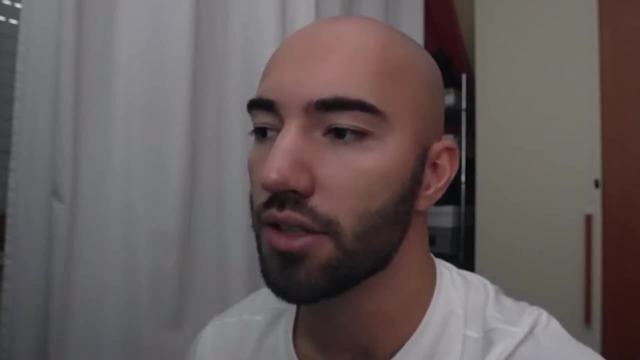 image like it's the same image of this picture right now. okay, so I'm going to. how to do is how to kind of search through this or at least compare a small number of images against our prompts, so that we can actually see which one of those images is the most similar. 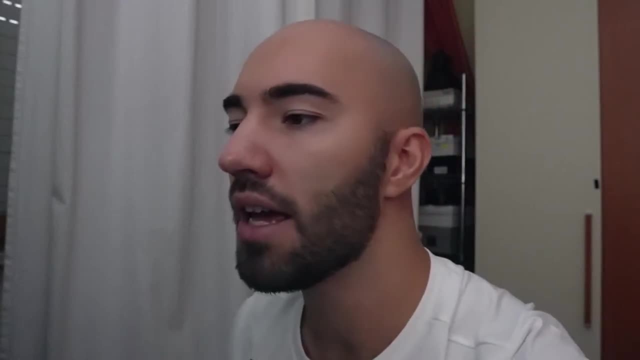 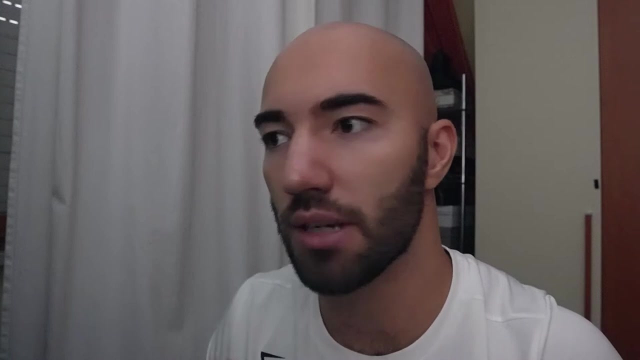 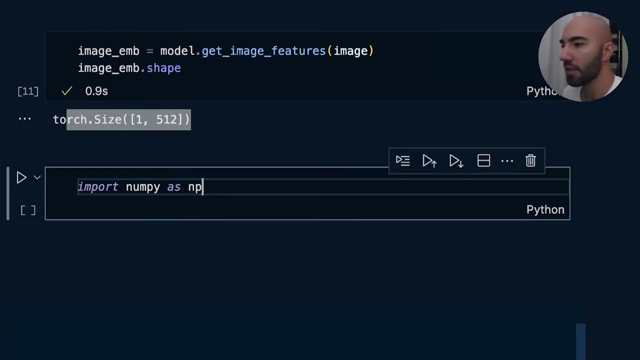 to a dog in the snow. okay, so to do that. we're going to want to embed more of these images. i'm not going to embed loads of them, just going to embed 100 images. nothing, nothing crazy. so we're going to import numpy as np, um, np, random seed. so this is just so you can replicate what. 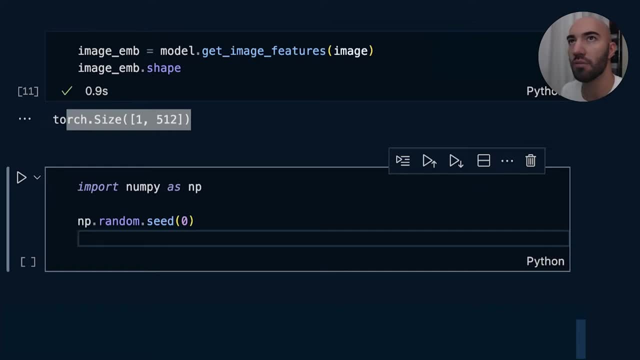 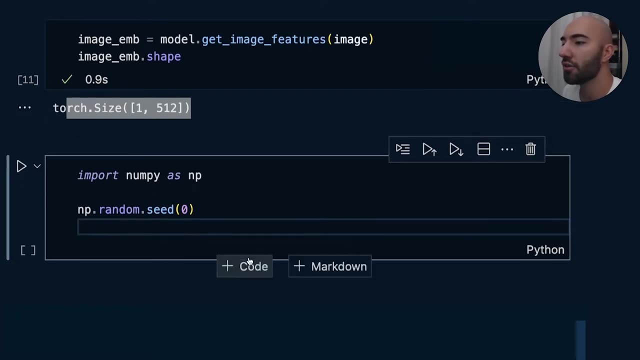 i'm doing, and so this will, this will randomly generate a set um set set of random numbers. okay, so the reason i'm doing this? because we want to take a sample out of the data set. we don't want to have the whole data set. i want it to be, at least, you know, somewhat random. so to do that, 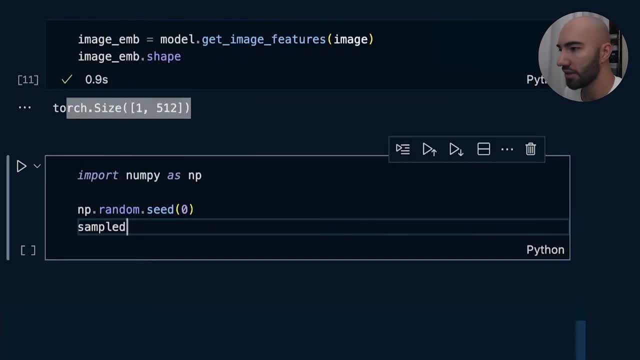 we want to go um. so sample indices are going to be equal to numpy random dot ran randint from zero up to the length of image net. it's actually plus one um and we need 100 of those, okay, and then we're going to convert. convert that into a list. 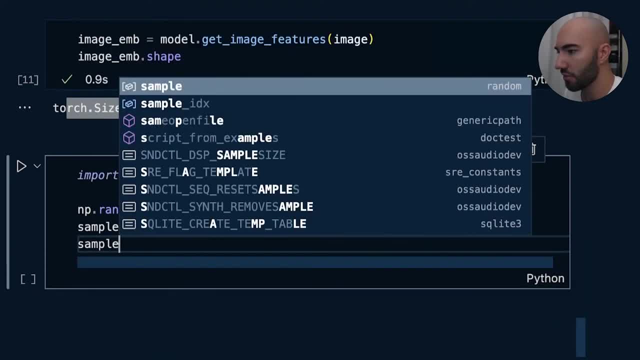 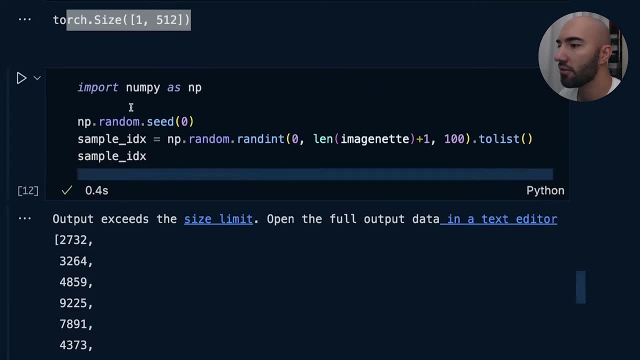 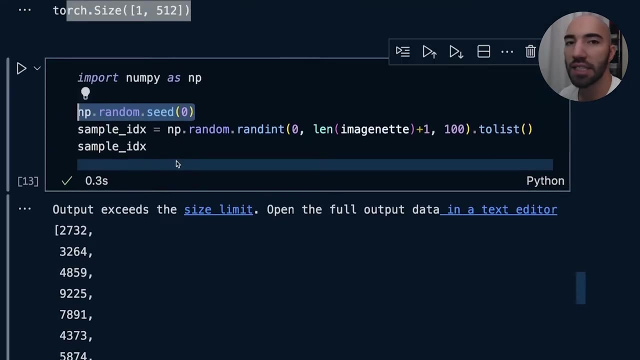 okay, um, i can maybe just have a quick look at what is in there. okay, so, just all of these, all these numbers here, okay, so, yeah, cool, and if we run it again, because we have that random seed set, the, the random set of numbers doesn't change and what i'm going to do is just create a list of 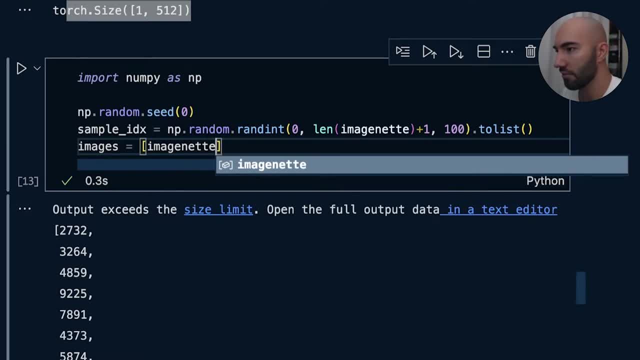 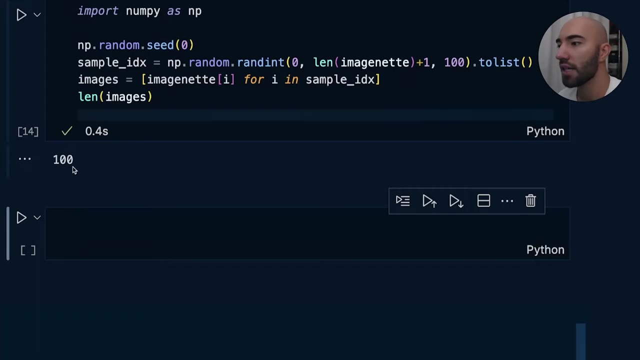 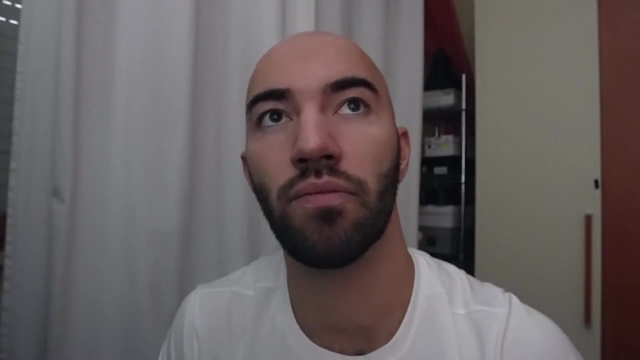 images. uh, using that, using those values. so i for i in sample ids, okay, and then we check length images, okay. so we now have 100 images from our data set and now we want to just go ahead and literally take everything we've just done and put into a for loop to create the embeddings for all. 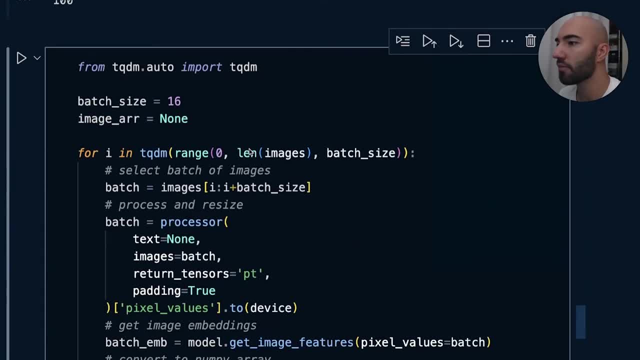 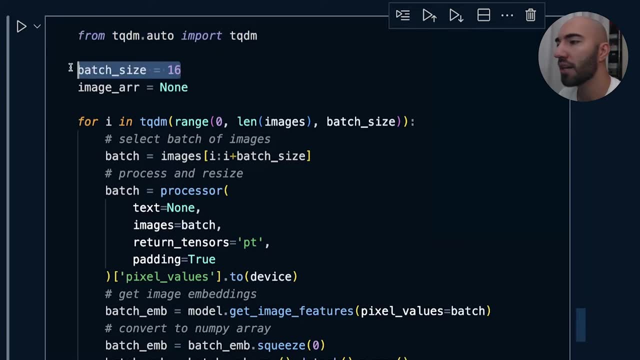 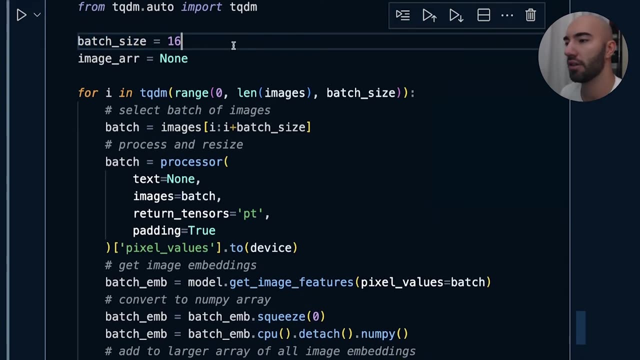 of these images. okay, so that will look something like this: uh, i'm using tqdm here. this is just a progress bar so we can see where we are. batch size: i'm saying how many images to perform this for in any one go. i can increase this. if you're on a, if you're using a like a bigger gpu or or whatever else, um, 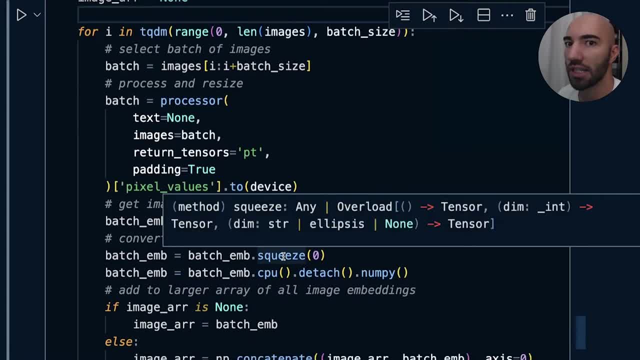 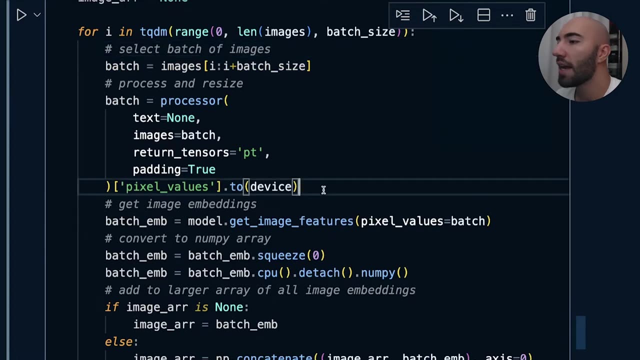 image array. i'm setting that to none for now. we we initialize that in the first and in the first loop, okay, and then we're just doing the same thing as before. so, except from this, um, so i'm selecting a batch of images based on the, on the batch size and then where we are processing and resizing the. 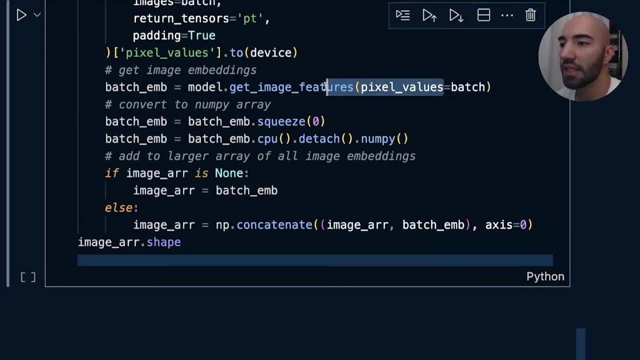 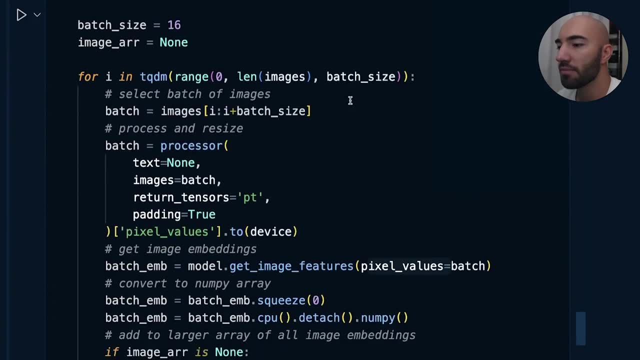 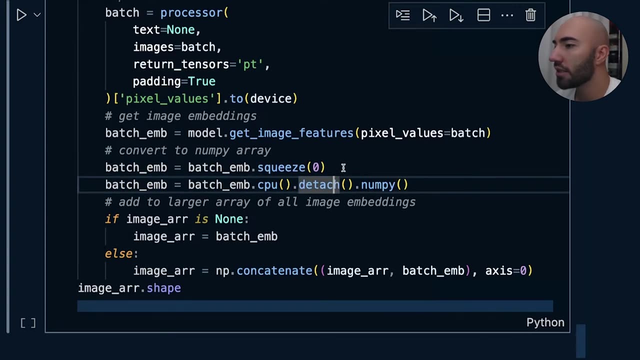 image from that batch, we're getting the image features. look exactly the same thing, i think, before. i actually didn't include pixel values, um, but it's the same thing. it's just a default argument converting into a numpy array. uh, did i show you this before? i don't actually think so. 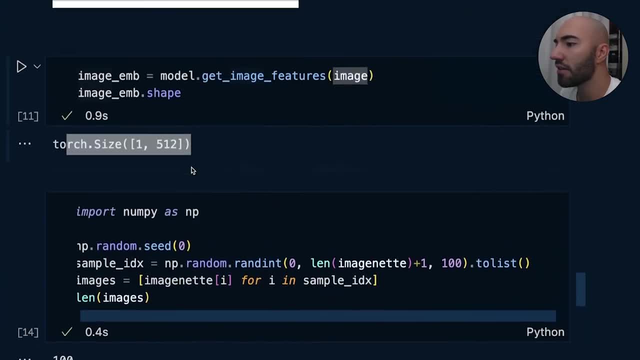 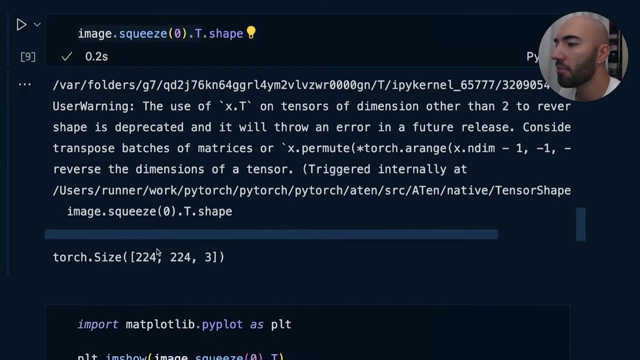 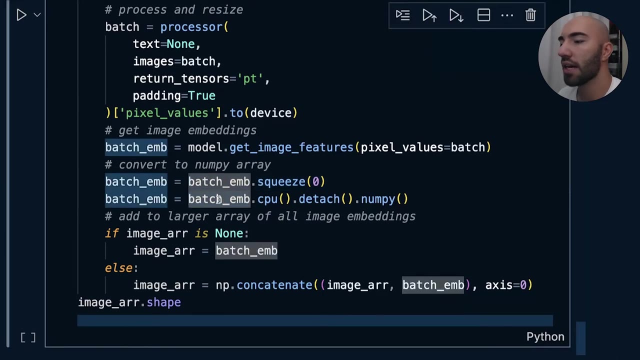 no, maybe not, but here the squeeze is very similar. it's the same thing as what i showed you up here. so we squeeze the first i mentioned out of that, like we did here, and then we are moving that batch of embeddings, uh, to the cpu, if it's not. 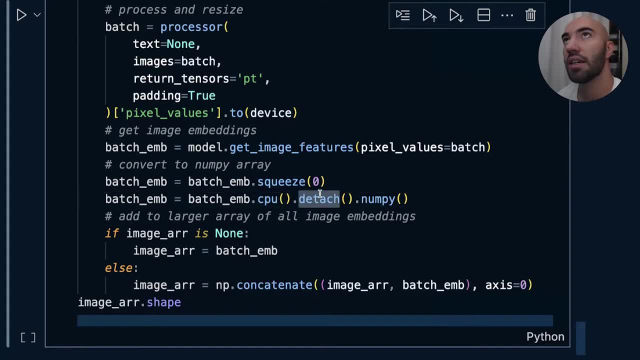 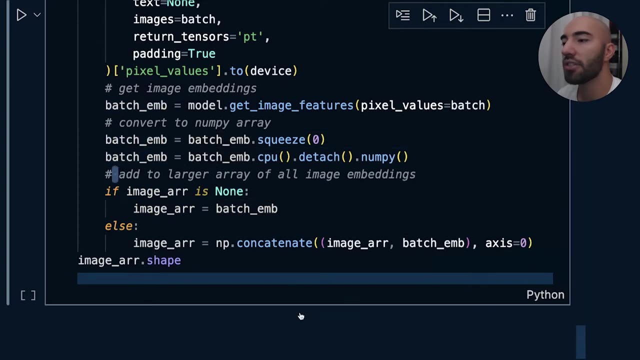 already on the cpu. uh, we're detaching it from the, the gradient, like the training graph um of pytorch, the pytorch model eg clip, and then we're converting into a numpy array. okay, and then i'm going to add that and that batch of embeddings to a large array of all image embeddings. okay. 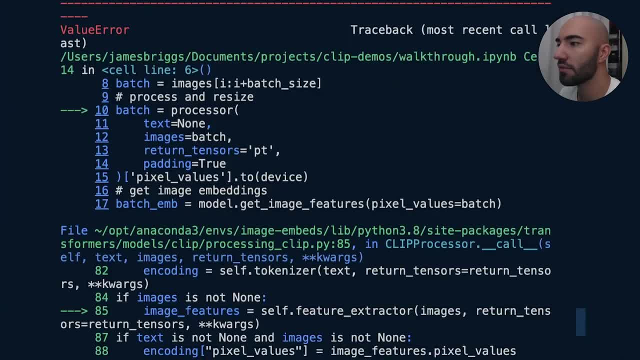 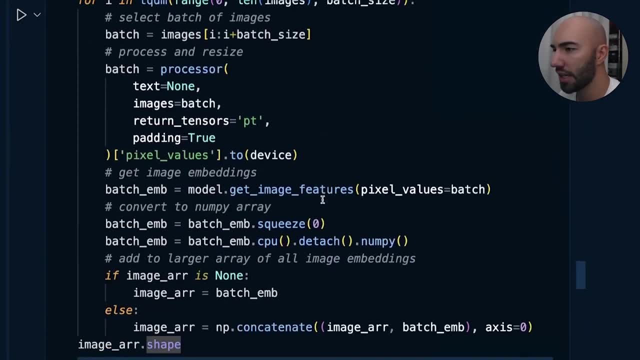 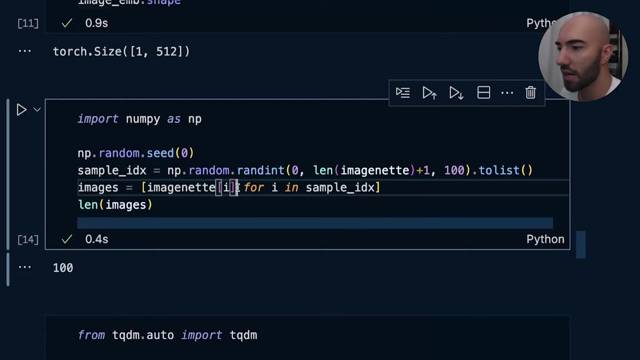 and that's that's why the, the image array comes in. okay, so let's run that. okay, so we come up here. i made a mistake in the code, um, so here i'm actually pulling in the, the full, like row or record at any one time. we don't do that, we want the image itself. 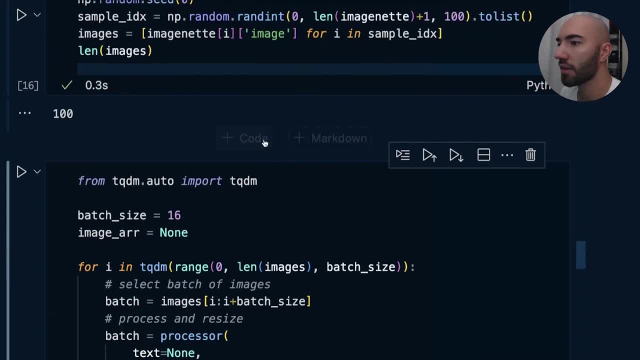 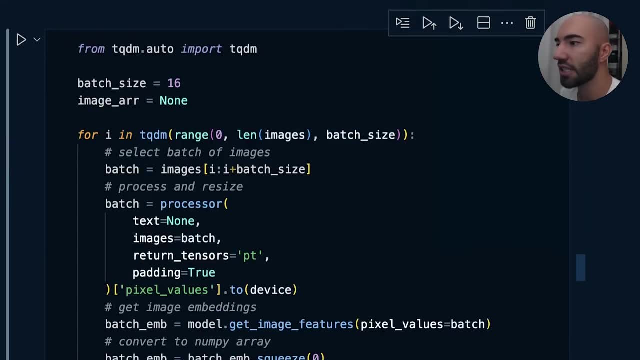 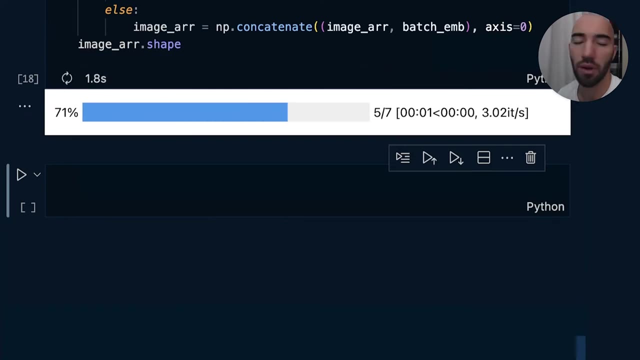 okay, so run that again. okay, and now, if we check the type of images, zero, we should. we should see, uh, it's a pill image. yeah, cool, we have pill here. now we can run this. okay, it won't take long. and now we have, uh, 100, 512 dimensional image embeddings. 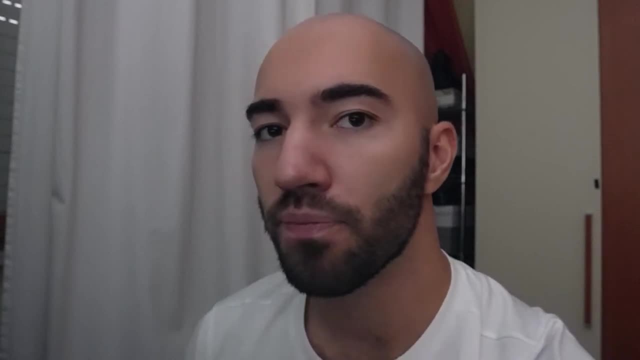 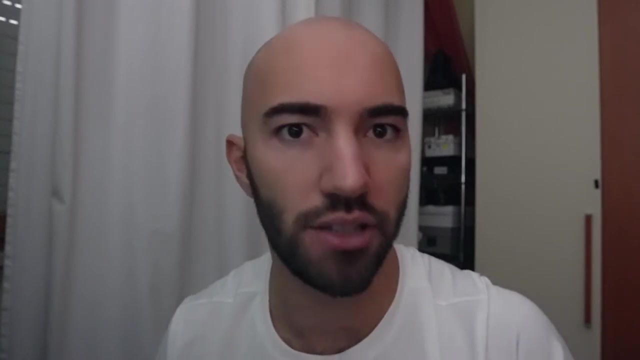 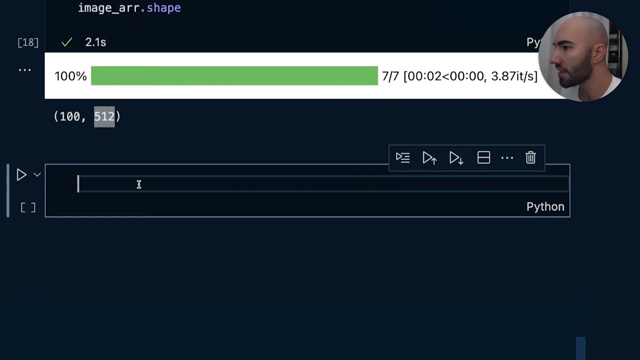 from our data set and we can now use them to compare to our initial text embedding and see which one of these matches most closely to that text embedding. okay, so i'm going to be using dot product similarity. so there's just one thing to to be aware of with that, and that is that it. 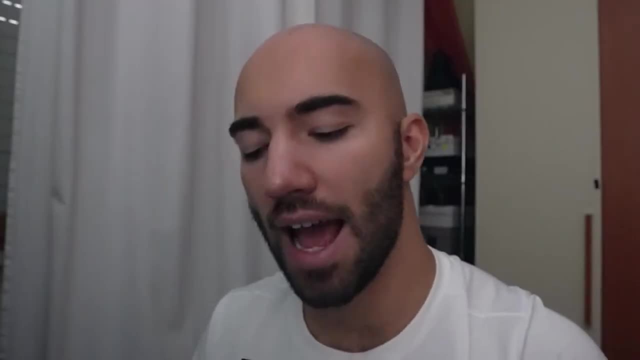 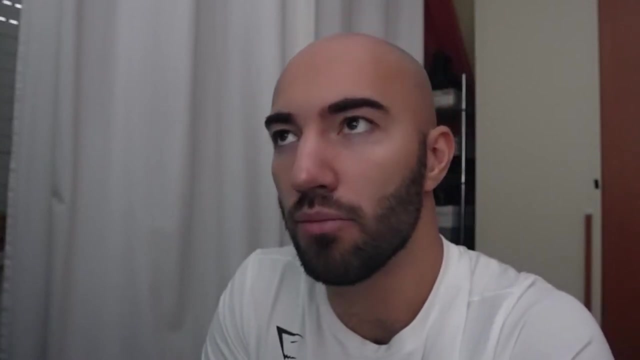 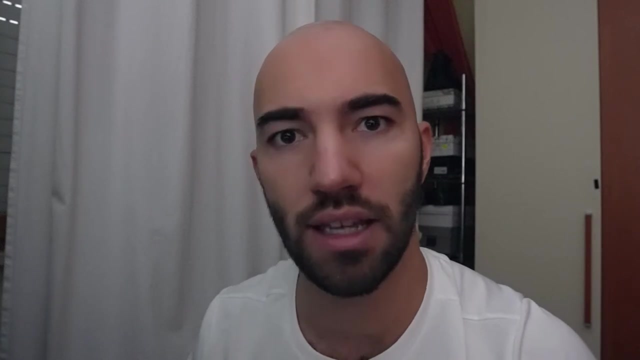 considers both the- the magnitude of the vector and also the angle. um. so in this case that will that can throw off our results, um. so we should normalize all of the image embeddings so that we are not um looking at the magnitude of vectors and we're only focusing on the angular similarity. 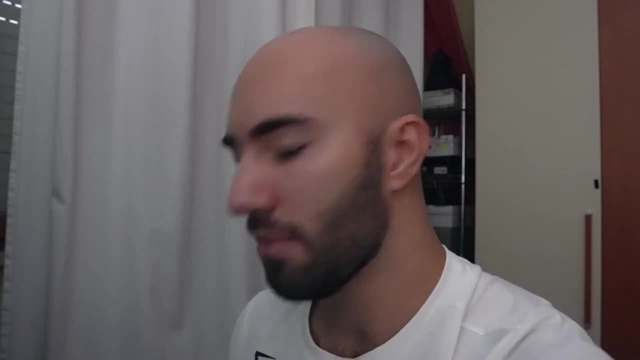 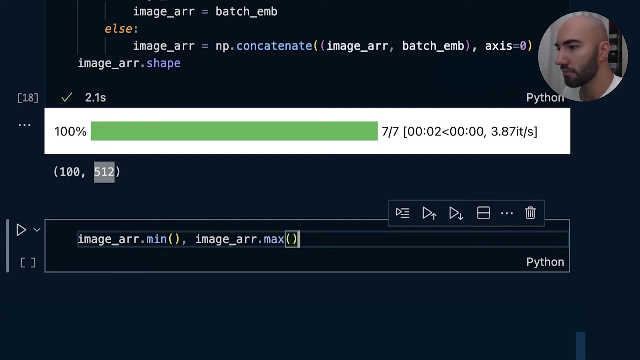 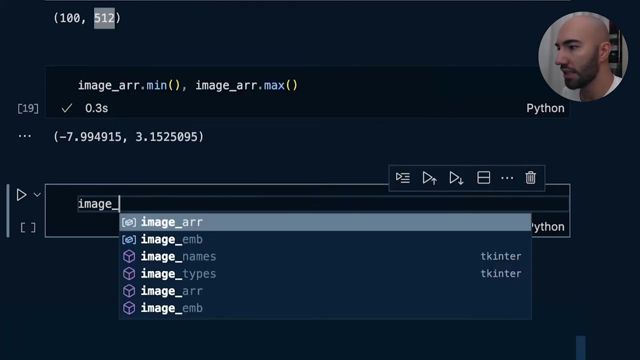 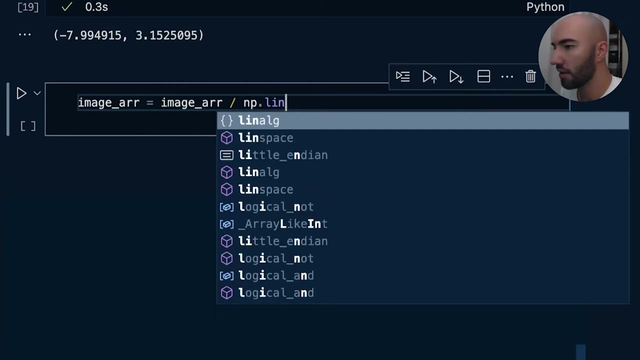 between our text embedding and these image embeddings now. so to do that we need to. i'll just show you quickly. um, so look at the minimum maximum. you know they're kind of all over the place. so to normalize we need to do this. so do image array divided by: do numpy lenaoge dot norm. and here: 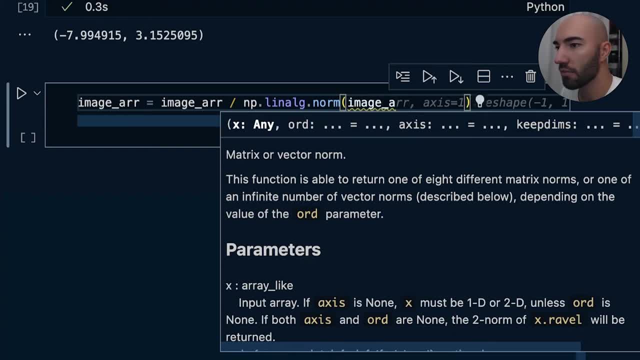 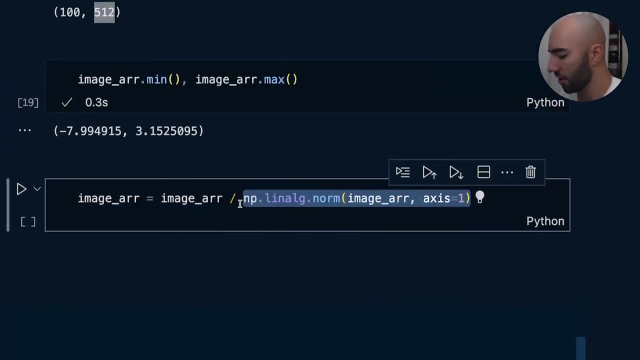 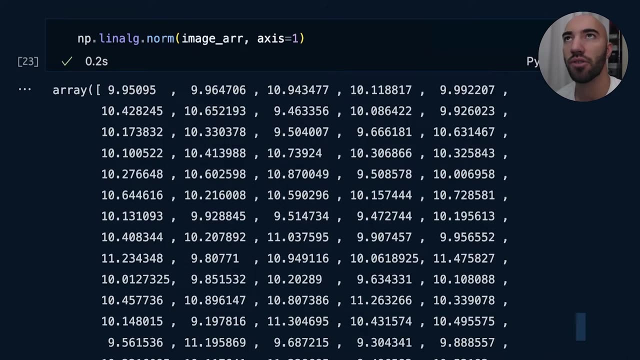 we have the um. okay, axis equals one, and let me i can show you what that is. so we have all these numbers and these are basically telling us, for each one of these vectors of what should we divide it by in order to bring each of them to within a um, within a set set um, within a set magnitude, pretty much um. 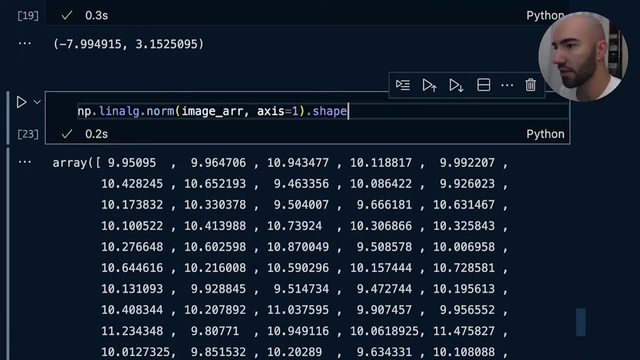 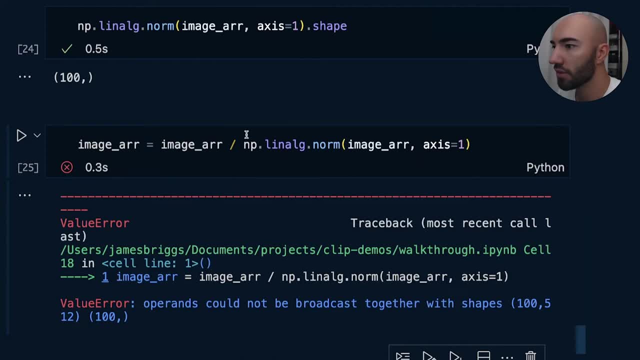 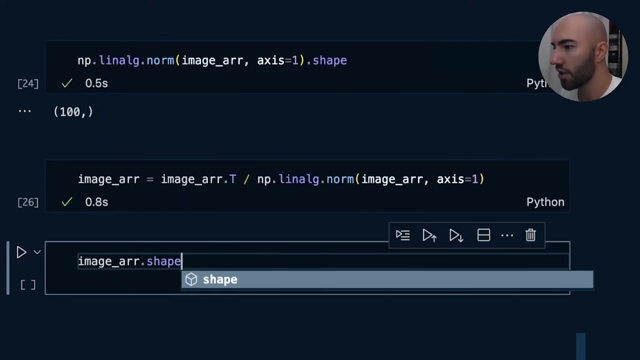 we can take a look at the shape. we'll be 100 um. so, yeah, we, we do that um. so i think i need to transpose this, okay and then? so the image array, the shape, is going to be transposed now, so i'm going to transpose it. 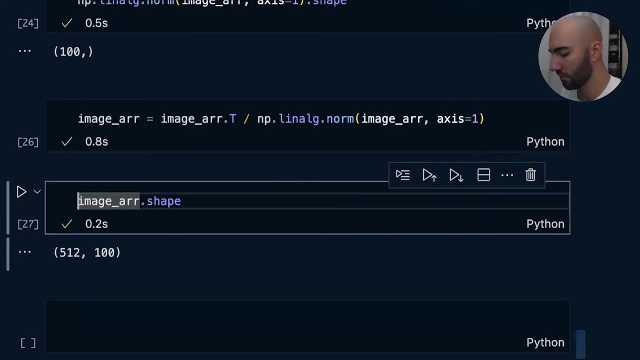 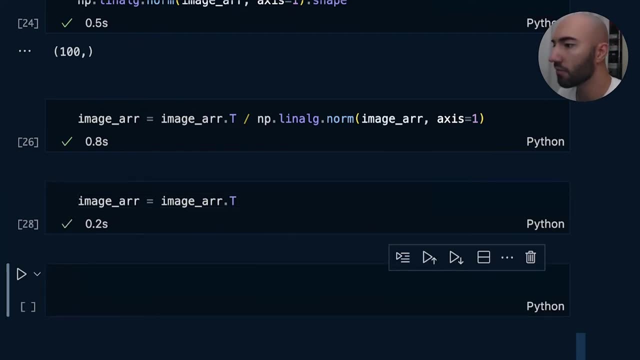 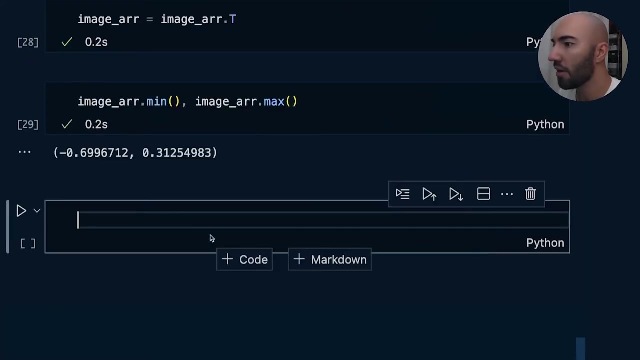 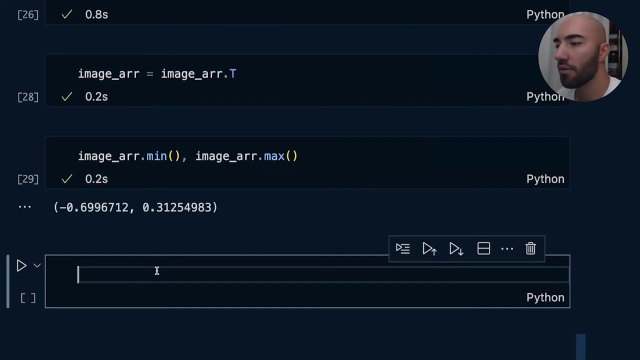 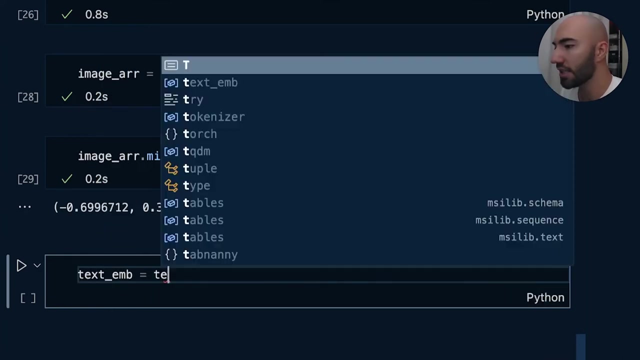 again: yeah, image array equals image array transpose- okay, cool. and now if we have a look at the minimum and maximum, so minimum and maximum, uh, we get these values uh, which are more reasonable, okay. so now what we can do is use dot product similarity to actually compare, uh, compare these. so text embedding: 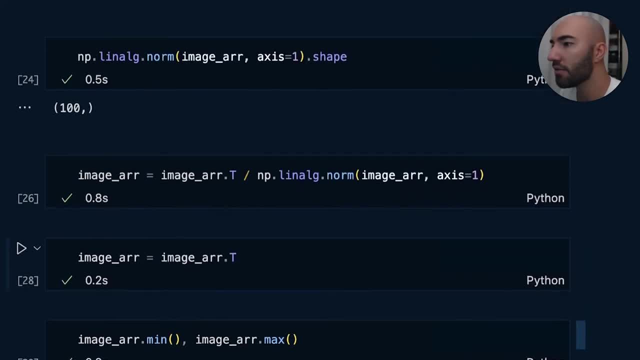 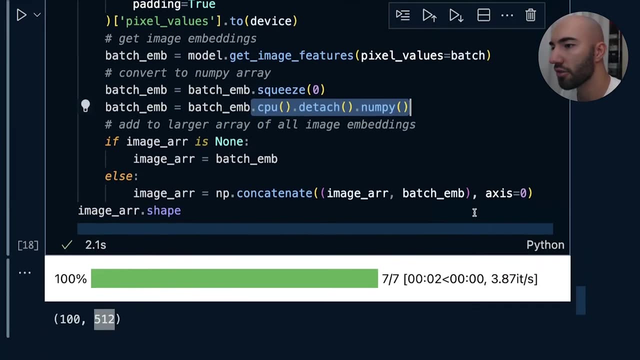 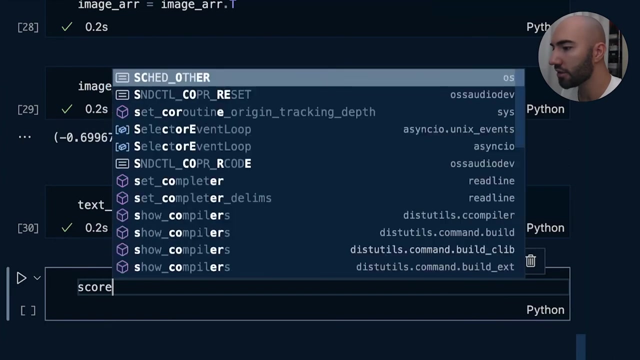 i'm going to take the text embedding and similar to before. what we did is we need to move it to the cpu, detach it from the, the pytorch graph, and then convert to a numpy array. okay, yeah, and then for the scores, uh, all we need to do is numpy dot and we are going to put the. 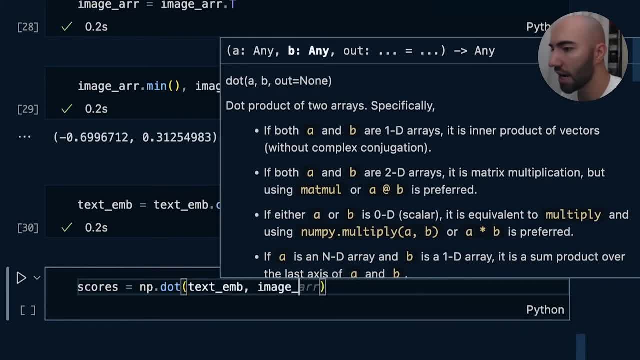 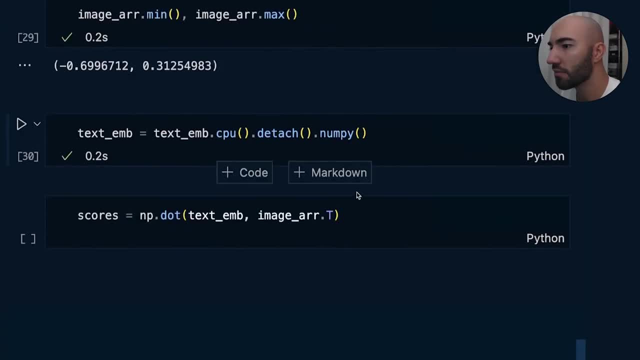 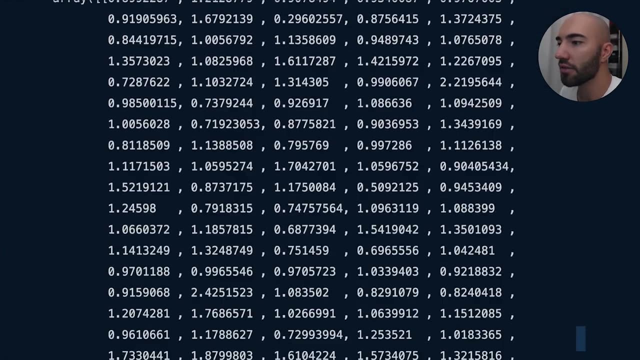 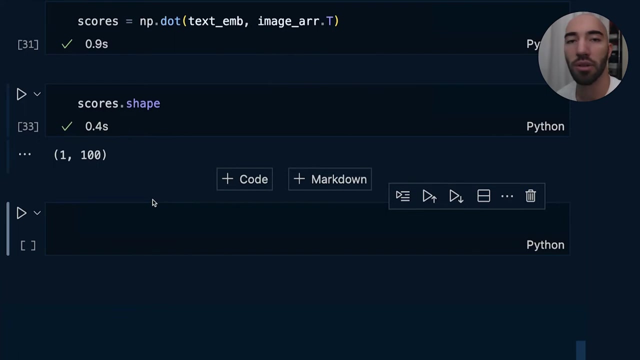 the text embedding, followed by the image array, and actually i think i need to transpose this again, so maybe we could have avoided transposing up here, okay, yeah, so the scores that we get here: we get a single score for every single vector, as we can see shape 100, and they are the dot product similarity scores. so what we can now do is: 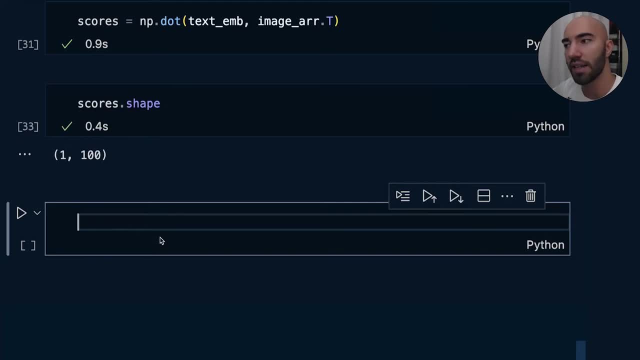 sort based on this scores array and just return, like the top, say, the top five images and see what the top five most similar images are for our particular, for our query. okay, so we're going to return the the top k. um, so top k is going to be the five most similar or the five items with the highest score. 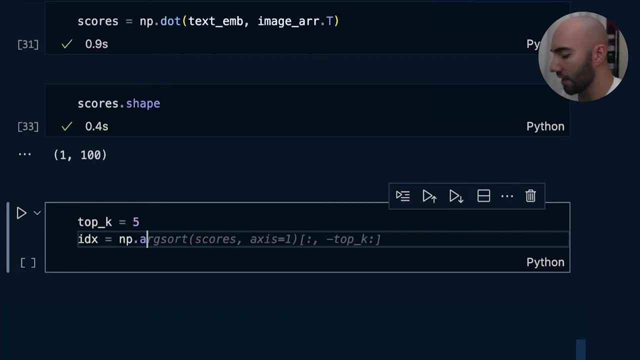 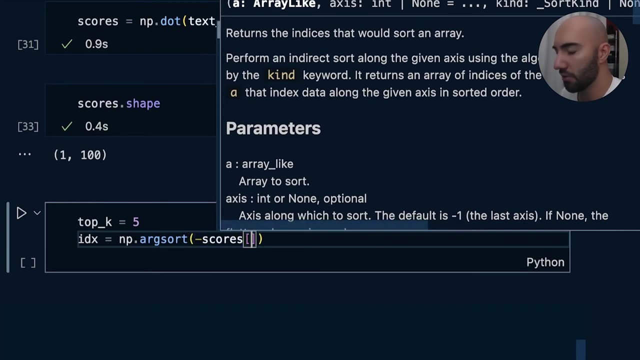 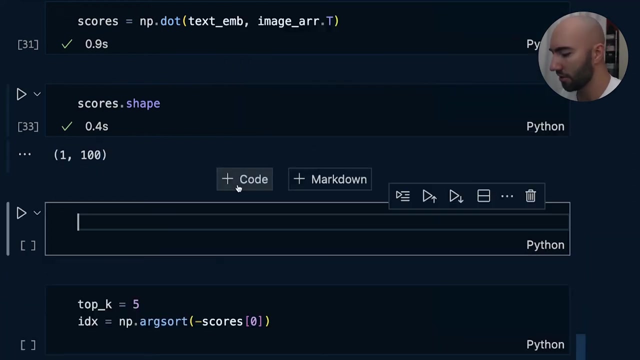 and then we want to take the index values using npx sort. we're going to add the negative of the scores there and just make sure we take um, because scores has this here. so we're, So we're actually just taking the. let me show you scores: 0.shape. 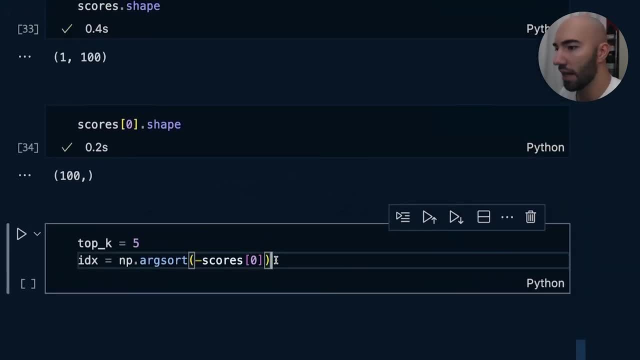 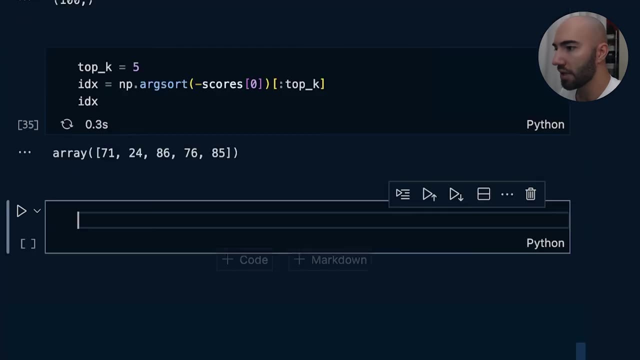 Okay, So it's taking the 100 values there, And then I want to take the top K from that. Okay, So what we're left with is these five index values, which are essentially indexes of the image embeddings and therefore the images. 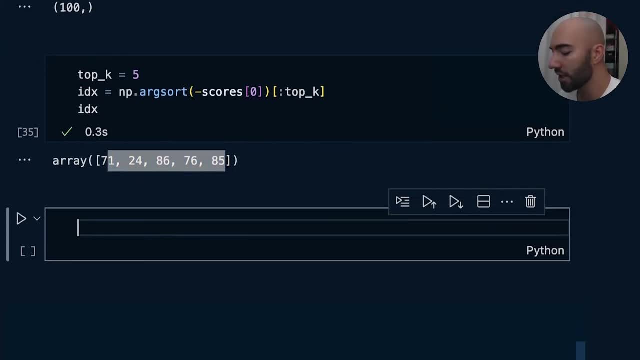 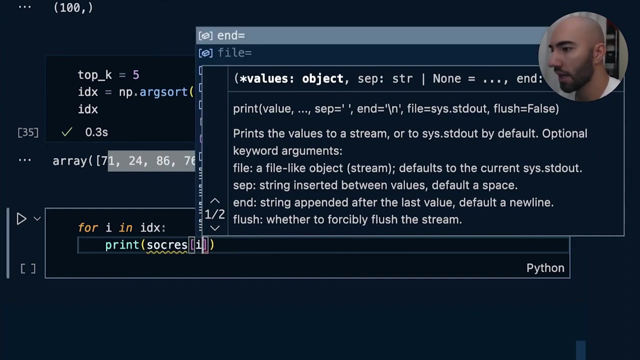 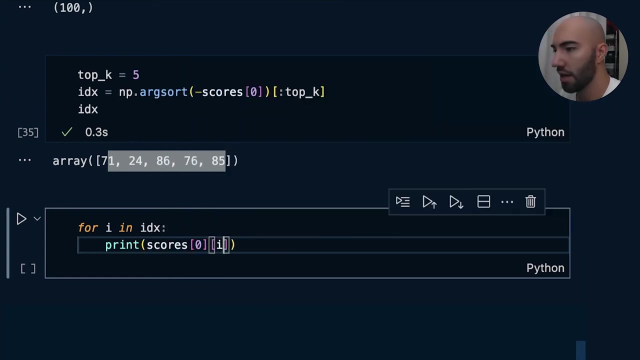 That are the most similar to our query. So we'll use matplotlib again to visualize those. So we do 4i in ID8.. Let's print the score first. So scores i, and actually that would be 0, i. 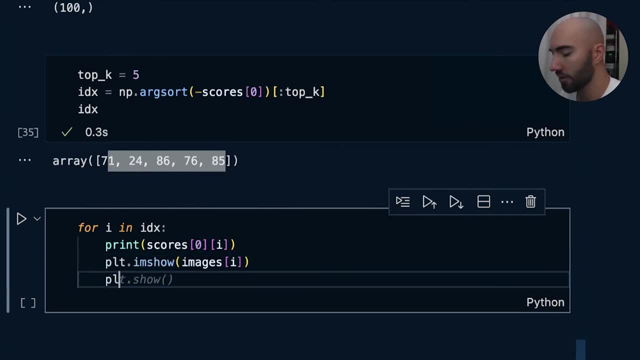 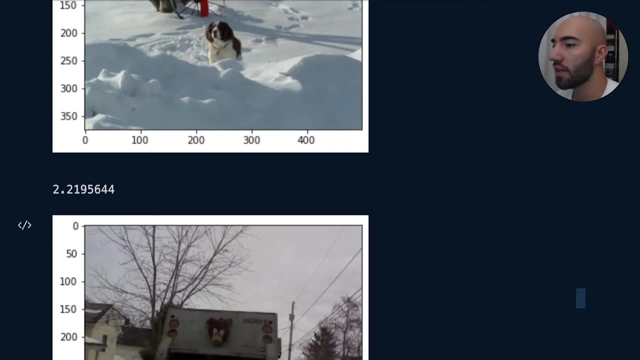 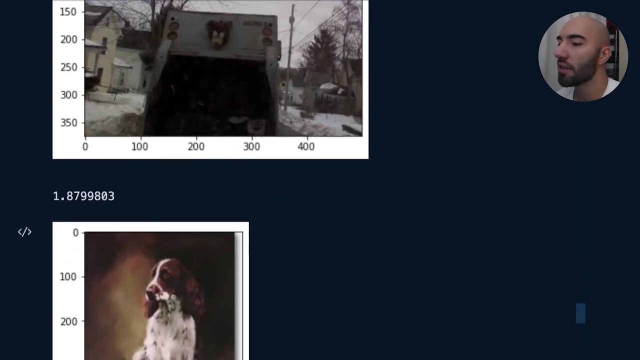 And then I am going to show, and I'm just going to PLT Show, Okay, cool. So yeah, I mean, that's it. So the first item, as we would expect, is a dog in the snow. So after that we get dogs and we get, like, these snowy areas. 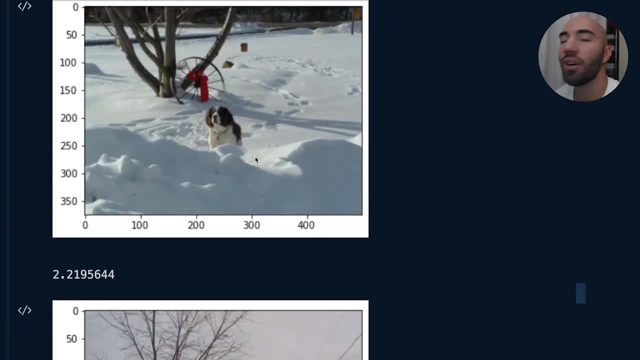 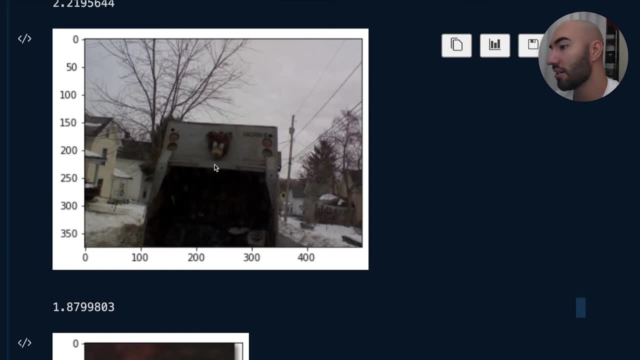 The reason for that is that we just don't have any more images of dogs in the snow. This one, I don't know what this is. It's like a toy that. maybe it's a dog, Maybe it's a bear, I'm not sure. 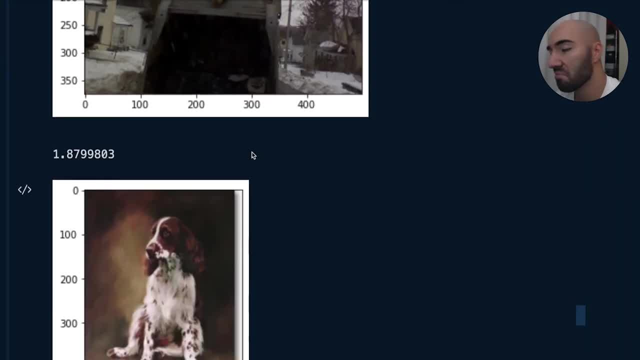 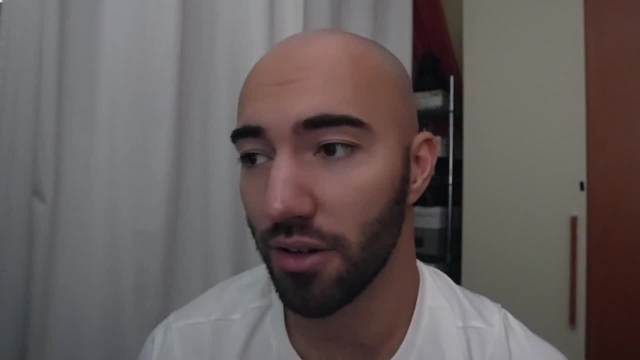 But I suppose technically that's like a dog in the snow. So we have that. So, yeah, obviously the model is performing pretty well And I think that's very cool that we can do that so easily. And yeah, I mean, clip is, I think, an amazing model that we can use to do a. 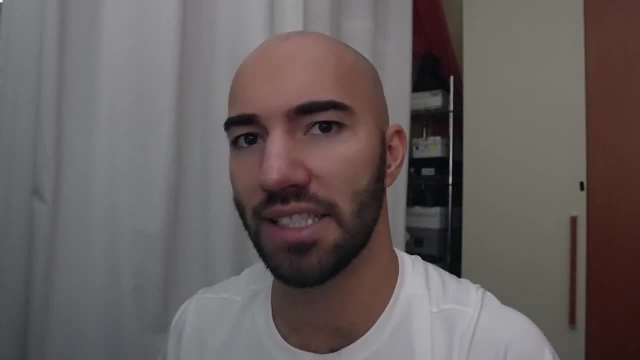 lot of cool things across both the text and image domain, which is super interesting, And it's definitely like, if you think just a couple of years ago this sort of thing was impossible and didn't seem like, at least not to this sort of degree of accuracy like. 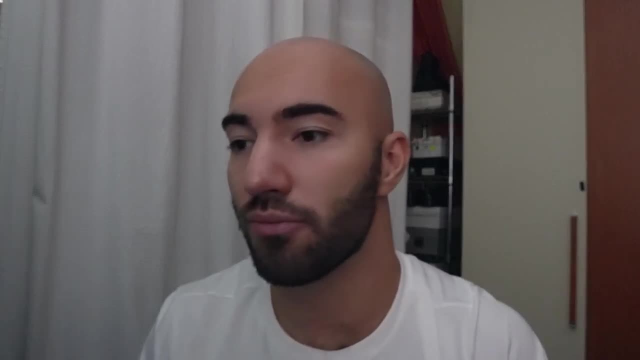 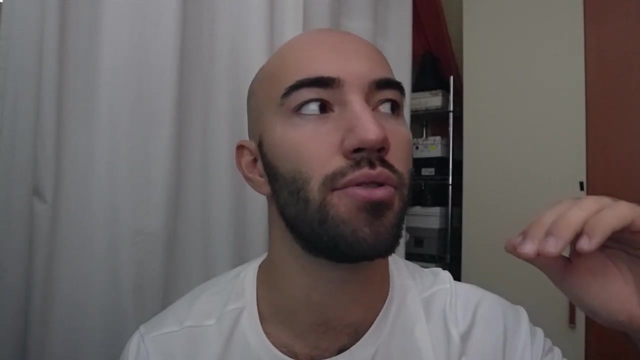 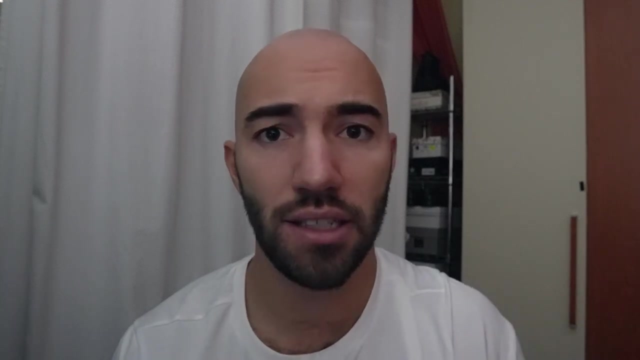 it was going to be happening any time soon. So this is, this is really cool. here We've obviously shown. I showed you how to do like a text to image search. You can do this like the deep. in reality, What we're doing is kind of searching through the vectors. 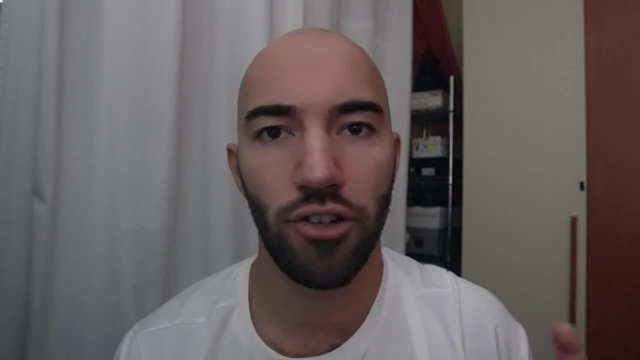 So it doesn't matter which direction you're doing that search. The vectors are all the same. So if you want to do a text to text search with with clip, you could. want to do image to image search, You could. if you want to do image to text or all of those things all at once, you could. 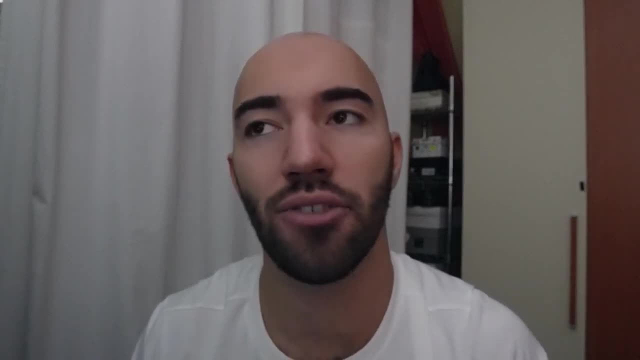 It's not, as you're searching through vectors, So what is behind those vectors doesn't really matter so much. OK, so I think that's it for this video. I I think clip is super interesting and I hope that you do as well in the future. 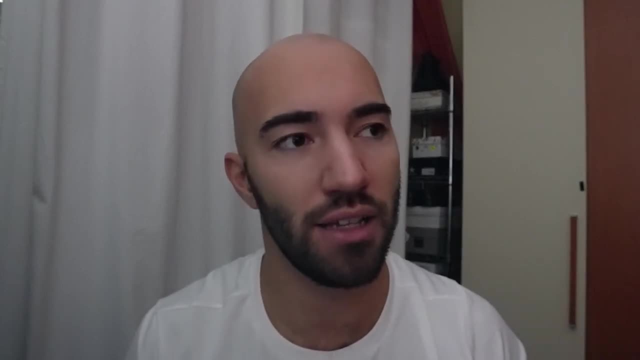 Or very soon actually. I'm going to be going into a lot more detail on clip. So if you are interested in that, subscribe and click on the little notification button and you will get a notification about that pretty soon. But until then, that's it for this video.